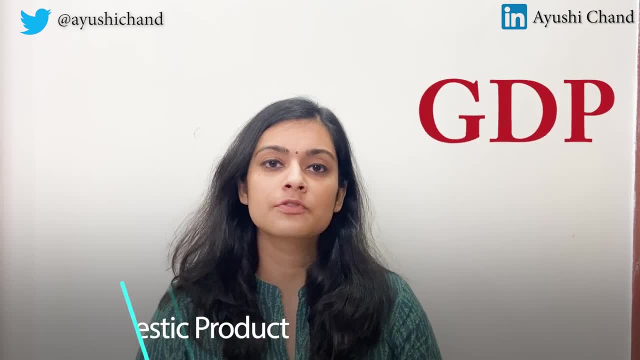 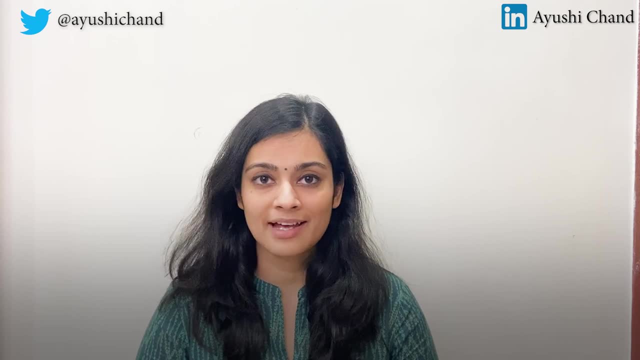 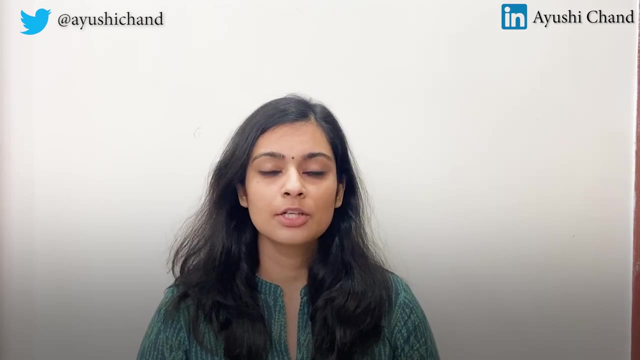 The Gross Domestic Product, or GDP, is one of the most frequently used economic terms. It forms the basis of all discussions that happen around economics, around finance, business or even public policy. However, it is also one of the most misunderstood terms. On this video, I'm going to break down GDP for you. I'll talk about what is GDP and what does. 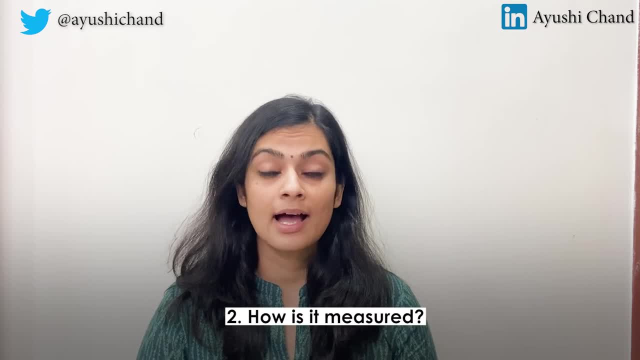 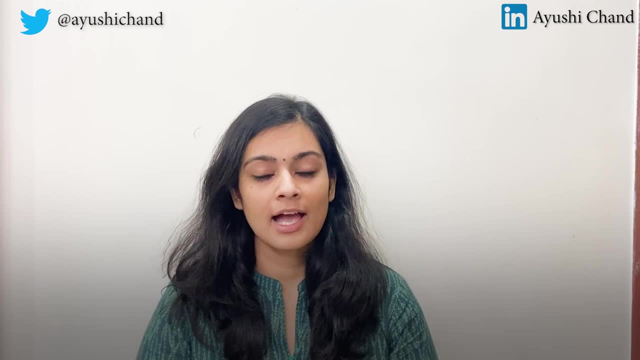 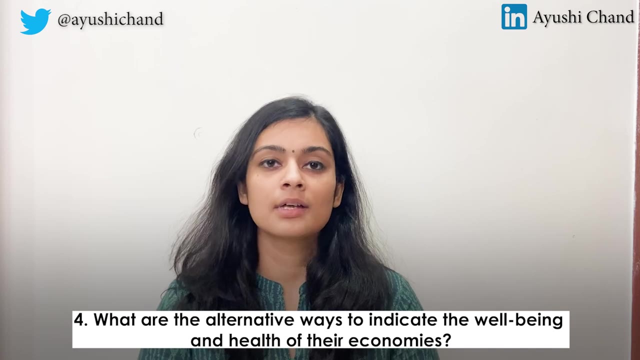 it signify. I'll also discuss how is it measured. I'll also discuss about whether it is a true indicator about the size or the well-being of an economy And finally, I'll discuss what are the alternative ways which countries have started adopting to actually indicate about the well-being. 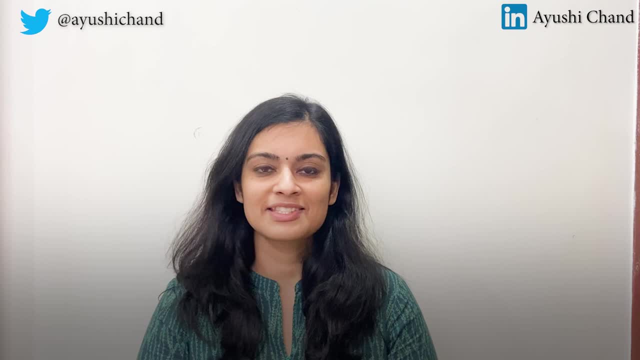 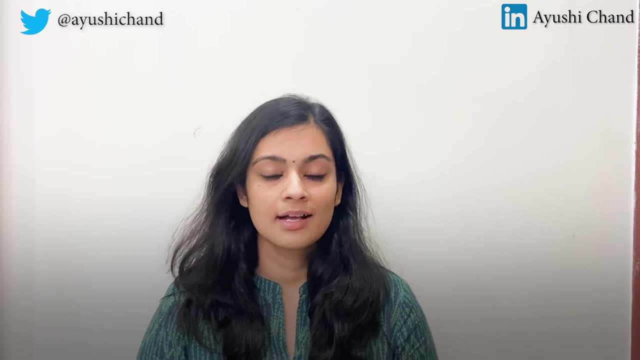 or the health of their economies. So, without further delay, let's start the video. Hello everyone, I'm Ayushi. I'm an Indian Economic Service Officer currently working with the Government of India. I have done my Economics Honours, as well as Masters in Economics and 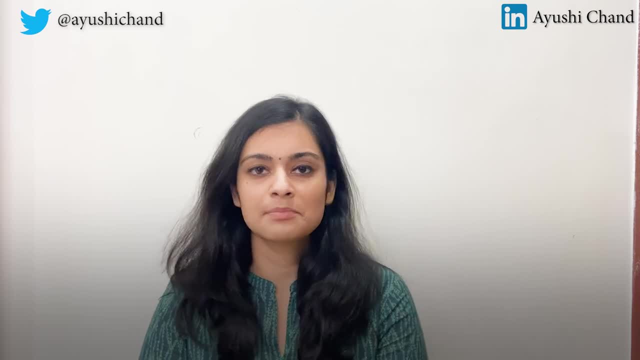 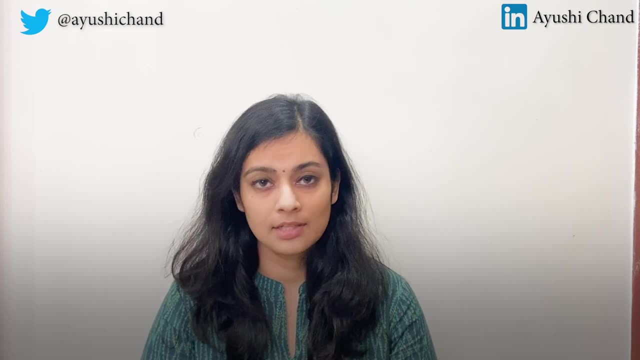 I've worked at the intersection of Finance, Economics and Business. I've also worked at the intersection of Finance and Public Policy for the last seven years. On this video, I'm going to discuss a very crucial topic, which is GDP. GDP forms the basis of all discussions which happen across business, across economics. 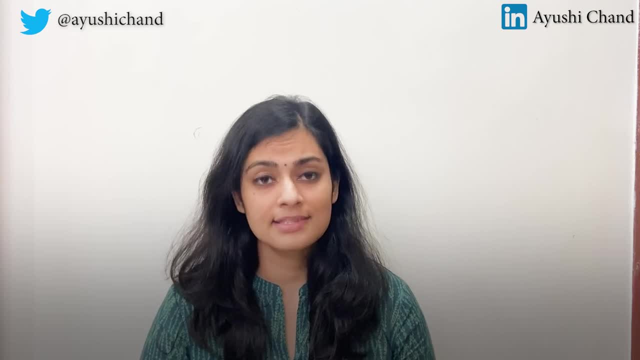 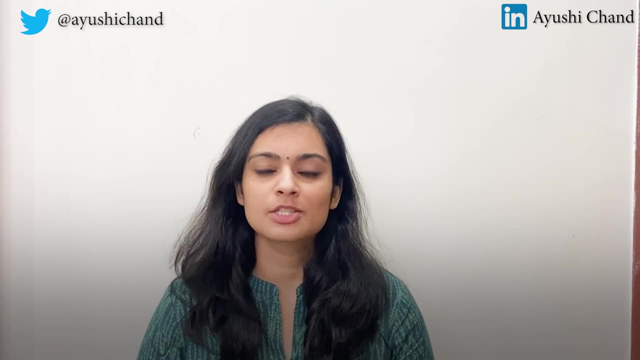 around finance and even public policy, And hence this is a concept we must be fully aware of and we must fully understand. So, without further delay, let's start the video. First of all, I would like to thank you from the bottom of my heart for all the support and encouragement you have been giving. 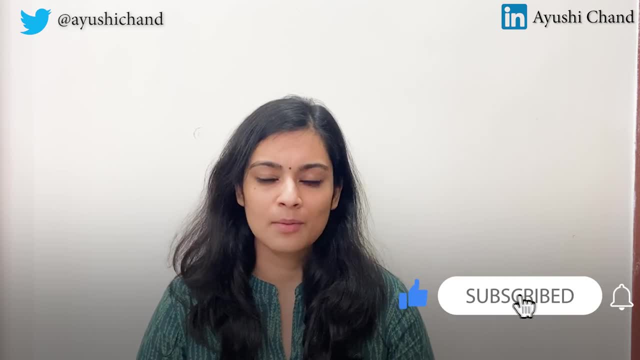 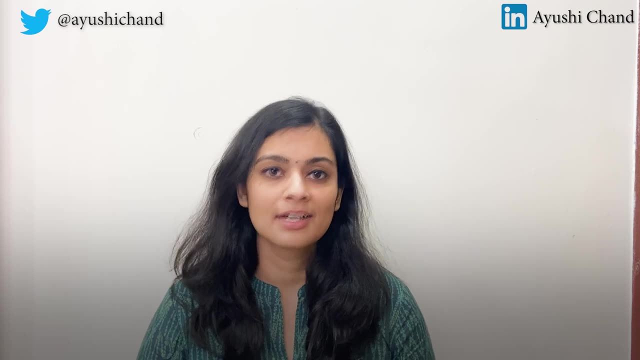 me over the last few weeks. I really appreciate all the likes, all the comments that you have given me. In fact, some of your comments have actually given me good ideas about what videos I can make to add more value to all of you, And hence I'll be working on those soon. Keep. 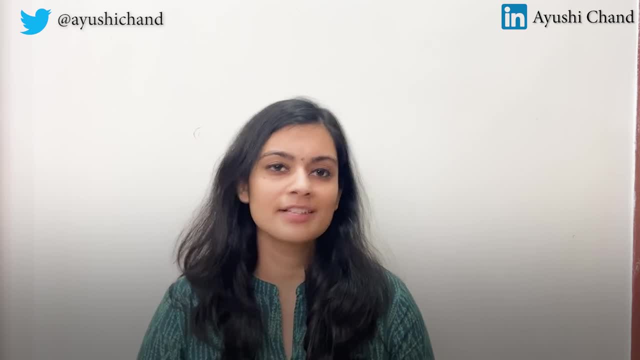 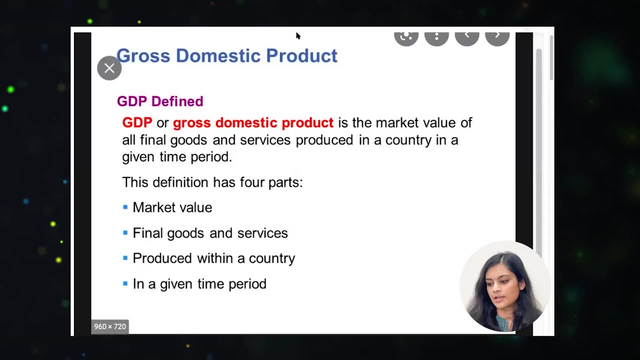 supporting, keep liking. It really gives me encouragement and gives me the confidence to make more videos. So let's jump on to the topic at hand, which is GDP. Let's look at the definition of GDP first. So if we look at the textbook definition of GDP, it goes something like this: 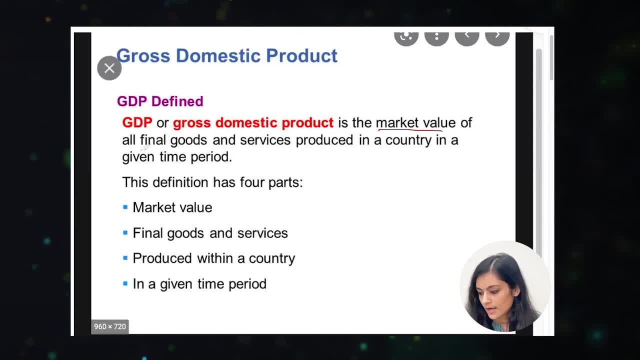 GDP is the market value of all final goods and services that are produced in a country in a given time period. Let's look at the four keywords. Let's start from the last one. In a given time period is quite clear. It means a specified time period, which means it could be a quarter. 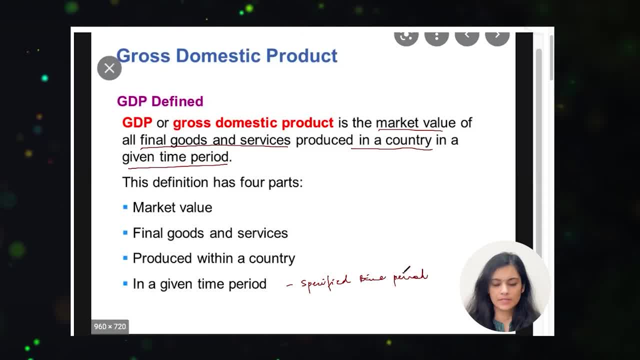 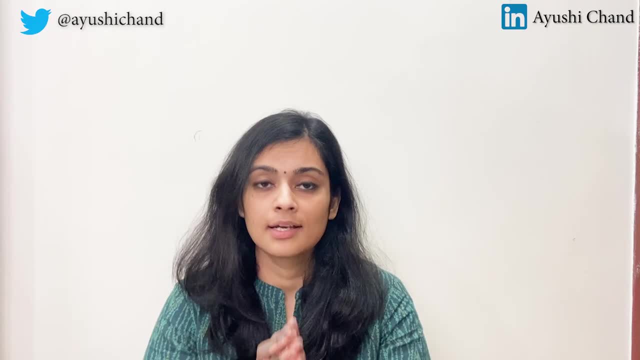 it could be annual, it could be two years, five years. whatever the specific time period is Produced within the country means within the national borders of a country. A good or item which is produced within the national boundaries of a country would be counted towards the GDP of the nation. Now it even includes islands such as Andaman and Nicobar. 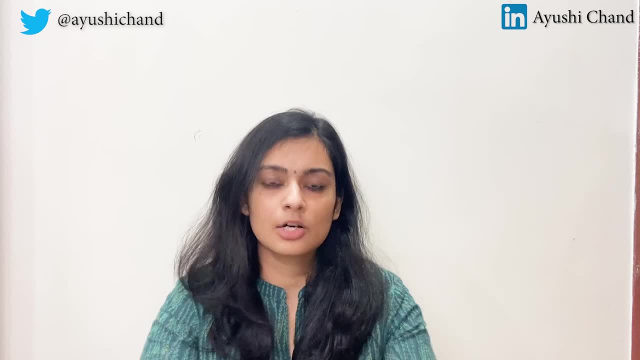 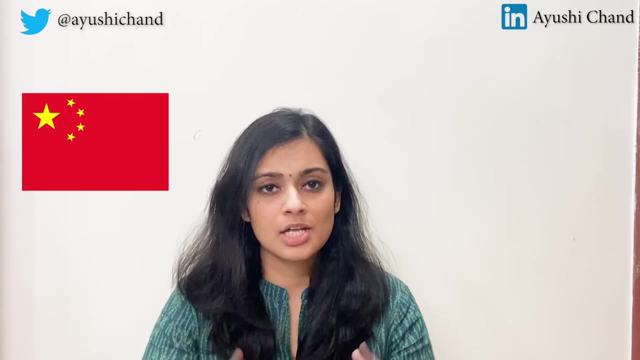 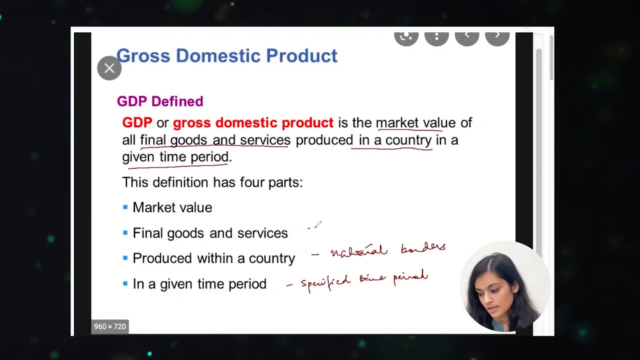 islands or the Lakshadweep islands, because these are a part of the national borders of India. A good which is produced outside India, outside the national borders, such as in China or in Germany, those would not be counted towards India's GDP. Final goods and services is an important part of 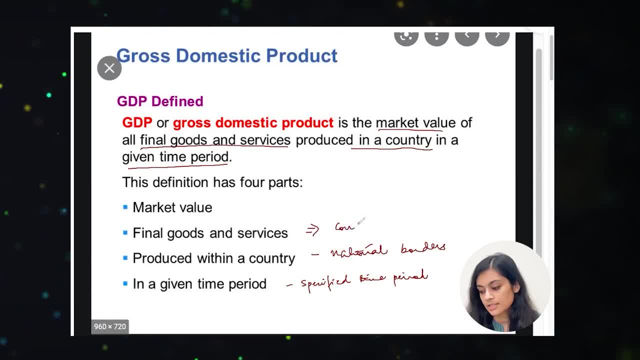 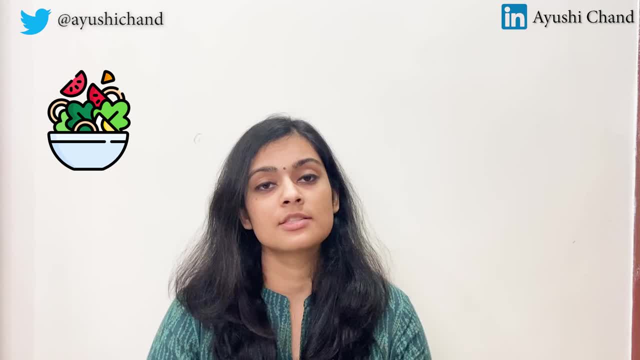 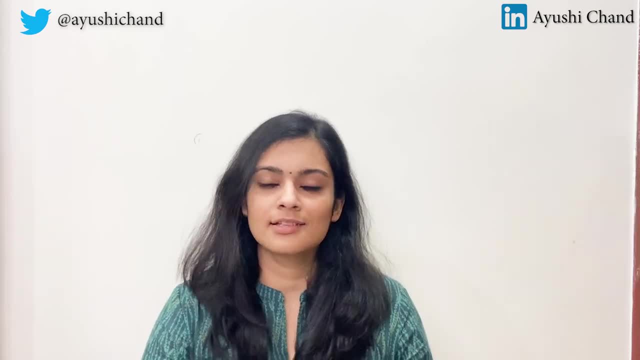 this definition. It means the goods and services that we, as consumers, are consuming, So it could be the household consumption, for example. we consume food items, we consume electronics, we consume education services or the health services. All these would be counted towards the GDP of the country, The market value. 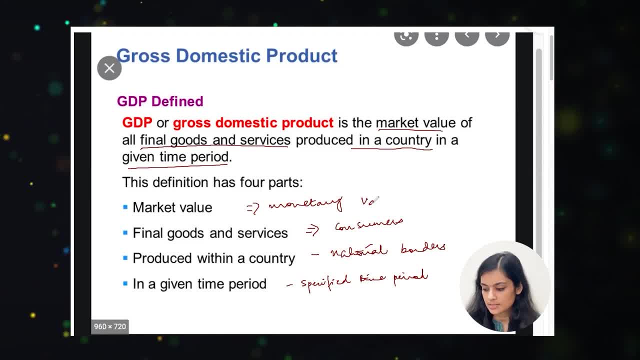 means the monetary value. that means all these purchases would be denominated in a particular currency. It could be INR, it could be USD. whatever the price is at which the goods and services are being sold in the market would contribute towards the GDP of the country. 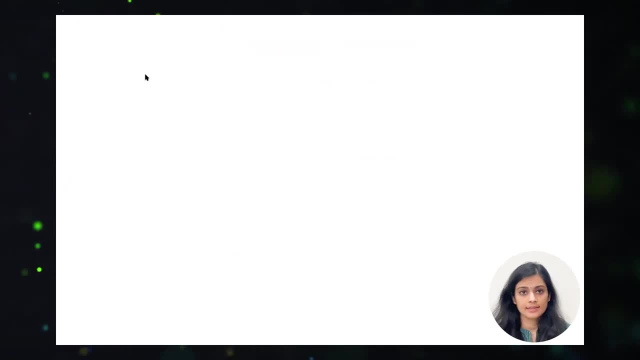 Let's look at an example now. Let's say that there is a basket of apples being produced, and this is the only good that is produced in the economy. So let's say there are only five apples that are produced Now. each apple is for, let's say, 10 rupees. 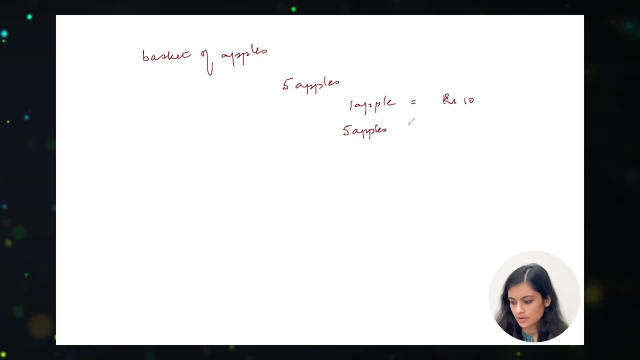 And five apples are for 50 rupees. Five into 10, which is equal to rupees 50.. Now, this will be the GDP of the country. This is the final product which are being consumed by the consumers, and this will be counted as the GDP of the country. Now, let's say that, besides, 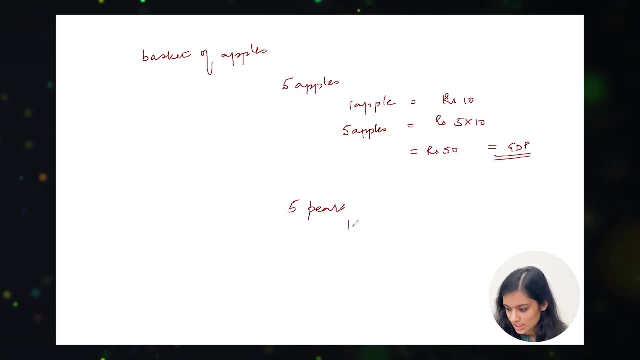 five apples, there are also five peers being produced. So each peer, let's say, is for rupees 50. So five peers would be for rupees 75. Now if we look at the total value of the final goods and services, that means the five apples plus five peers. This rupee is 50 plus rupee 75. 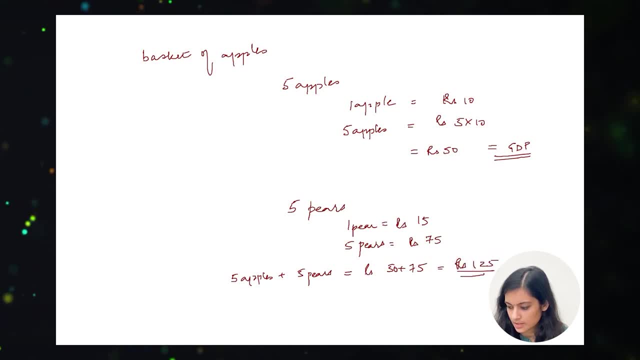 which is equal to rupees 125.. So this becomes the GDP of the economy, where only five apples and five years are being produced. This is a very, very oversimplified definition. I hope you understood it. This is actually a class 10th or 11th definition, and I just 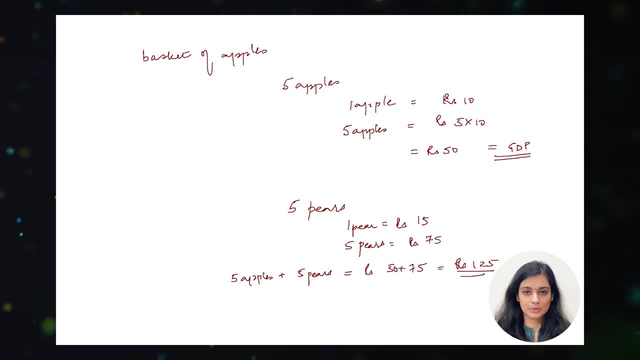 gave it to give you a view of how GDP is calculated, but I'll go on to more technical details of it when I discuss how is it actually measured? But what does GDP signify? Let's say that the final value of all goods and services that are produced in an economy in year one is US dollar 10,000.. Let's say in: year two it increases to US dollar 15,000.. This means that there is an addition or an increment of US dollar 5000.. Now what does this $5,000 signify? This means that $5,000 worth of goods and services were produced in the 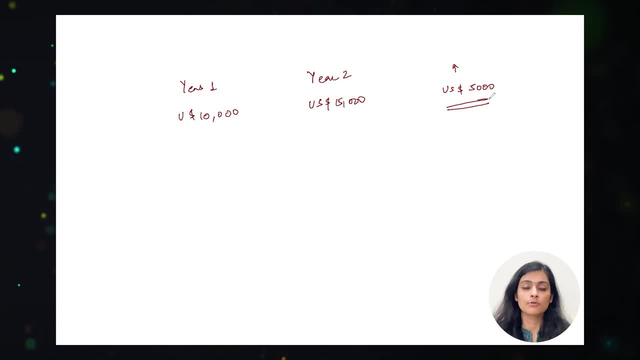 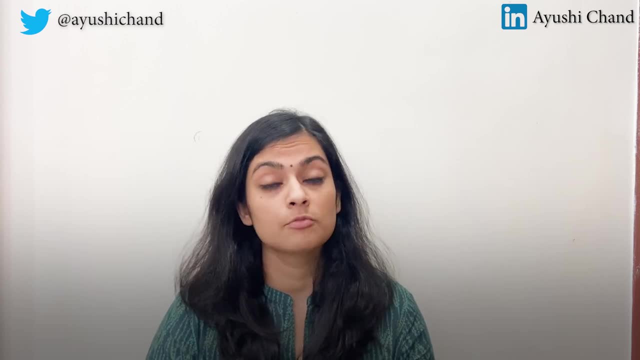 economy. This also means that there must be a demand for this much worth of goods and services. Think about it this way: Why would companies and factories produce more goods and services? They would produce more goods and services only when there is an adequate demand in the market. If there is no demand, they do not have an 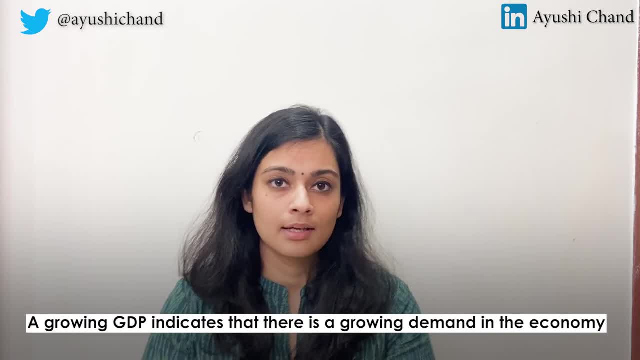 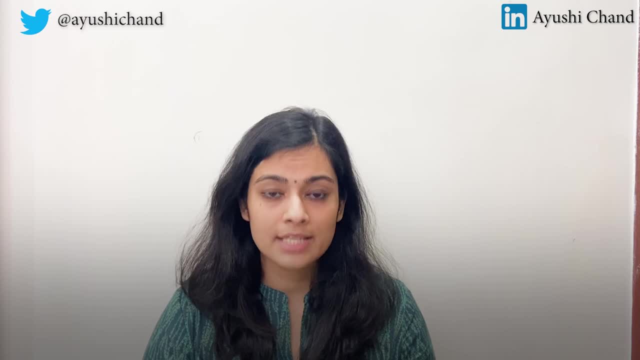 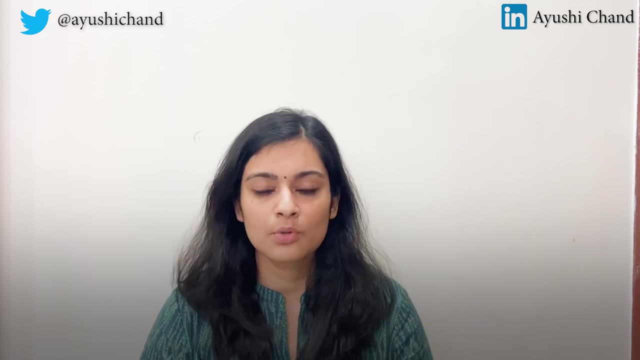 incentive to produce. So a growing GDP indicates that there is a growing demand in the economy. That means people are demanding more. there is also an income rise. they have spending power, they want to purchase more goods and services and hence factories and companies are producing more goods and services. Hence, 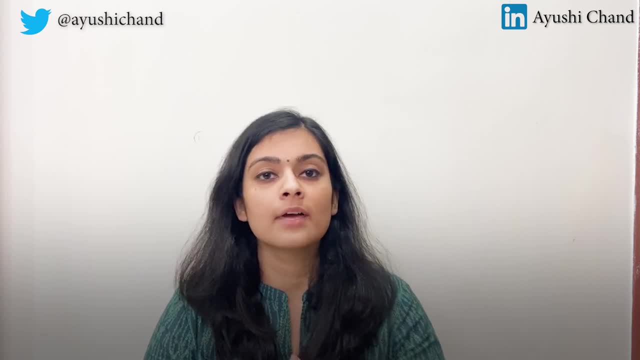 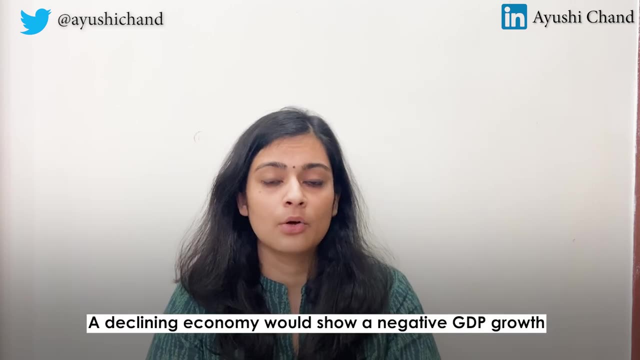 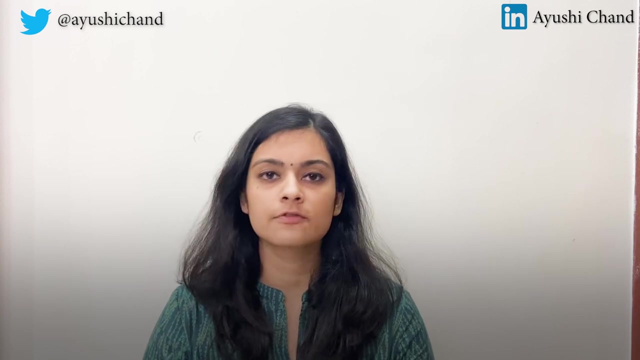 GDP is considered to be an indicator of economic growth. A growing economy would show a positive GDP growth. A declining economy, on the other hand, would show a negative GDP growth. For example, when the pandemic hit India in 2020 and there was the first lockdown, there was a decline in spending. People were saving their 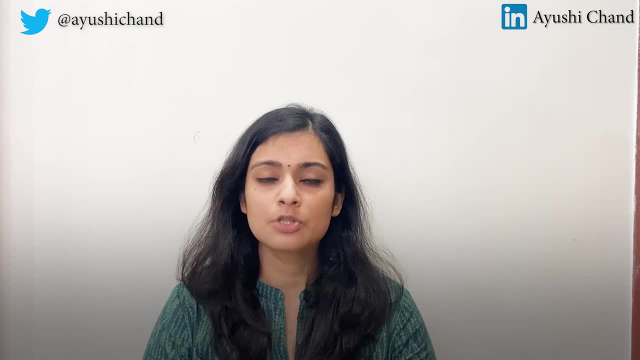 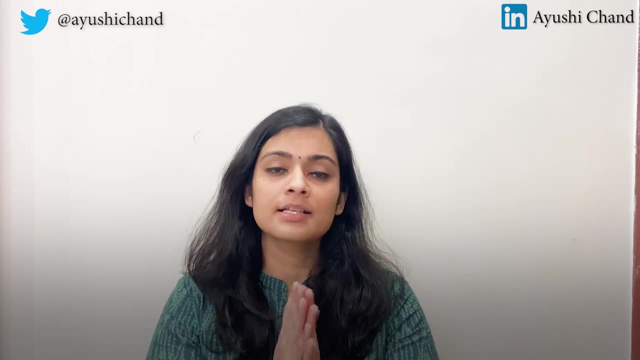 money. they were only purchasing essential items. they were not consuming other things, such as electronic durables, or they were not going out. they could not travel and hence the spending had declined. This is also a topic which I discussed in the first part of 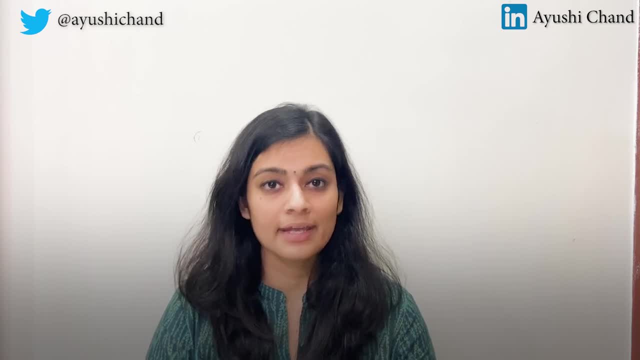 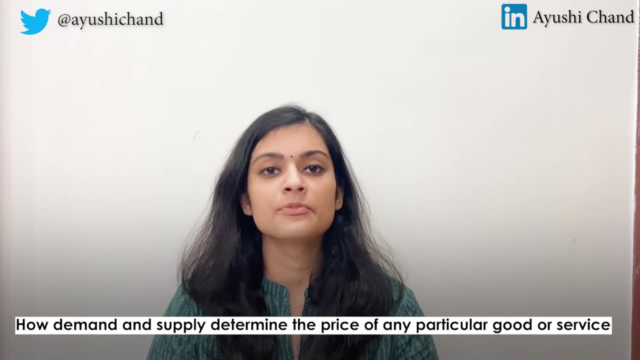 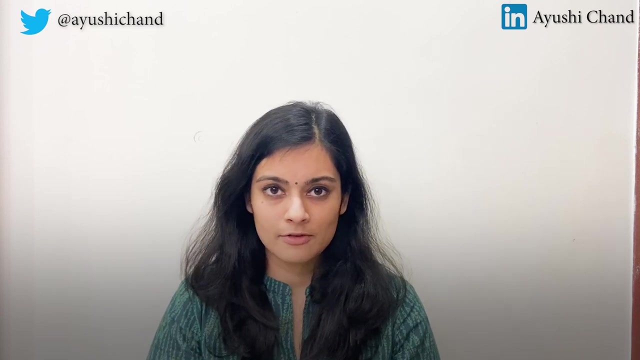 this economic series that I have been making for you about demand and supply, I discussed how demand and supply determine the price of any particular good or service in the market. So you must watch that video because that forms the basis of all that happens in the economy. So if you haven't, 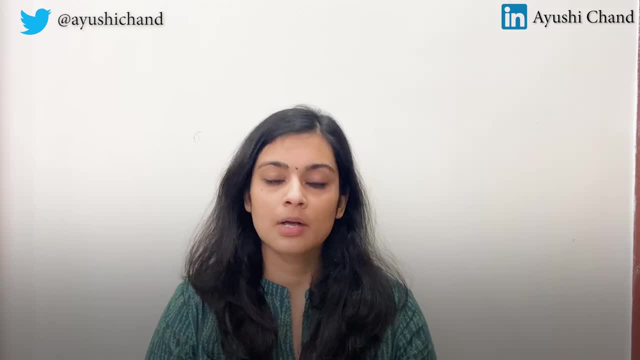 watched it already. I have linked it on the top. Do go and watch it right now. So, coming back to the story in 2020, when the pandemic hit India and there was a decline in spending, companies were shut down, a lot of factories were not operating, people had lost their jobs, unemployment was at 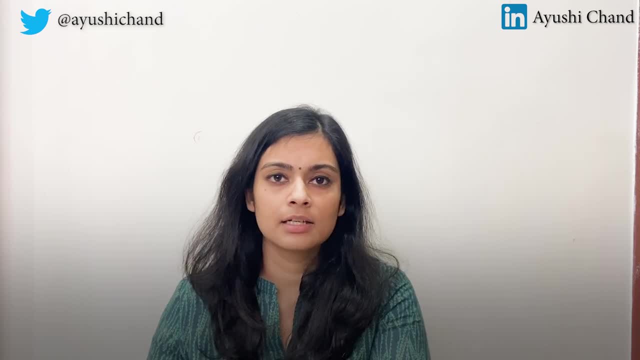 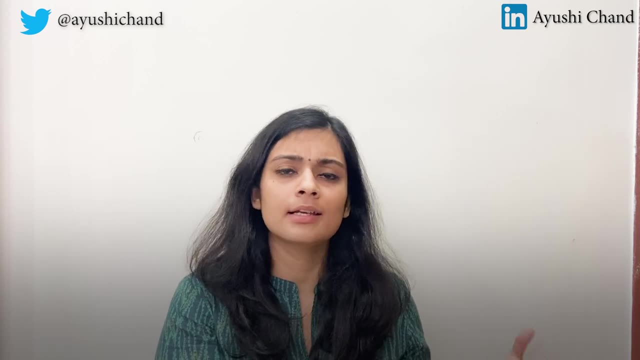 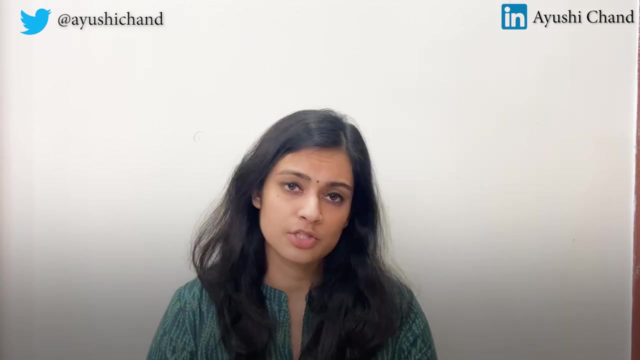 an all-time high and, correspondingly, because there was a decline in demand. even companies and factories which were actually producing goods during that pandemic also did not find an incentive to produce goods and hence the GDP contracted. Now GDP contraction is considered to be a dangerous sign. A GDP contraction for two? 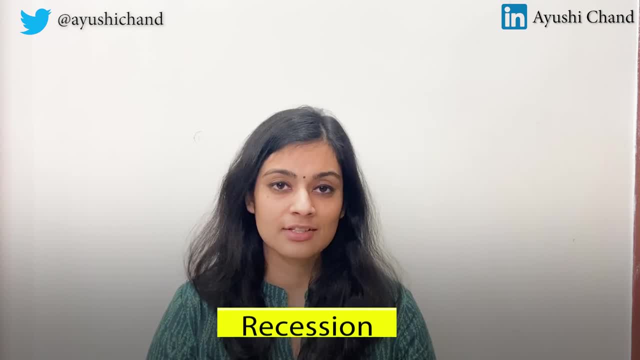 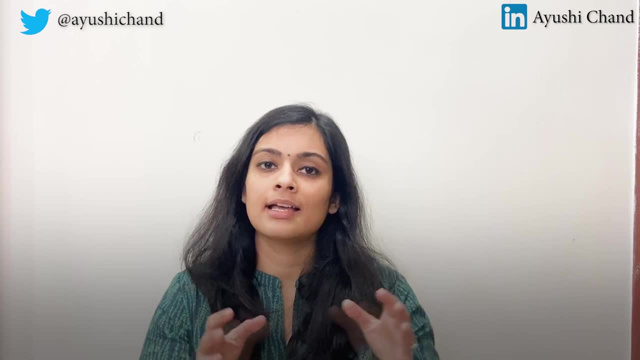 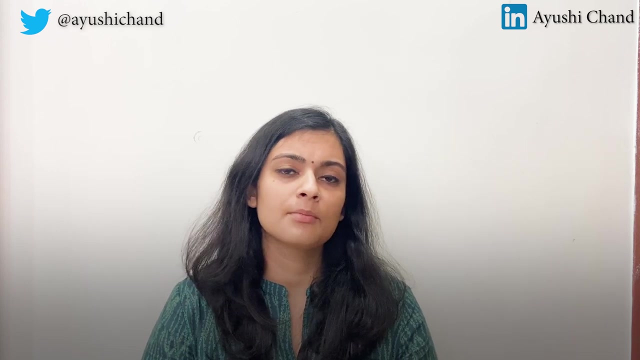 consecutive quarters is technically called as recession. So if you see that GDP has contracted for one quarter and the next quarter, then technically that economy is in recession With me so far. So this is what GDP is and what it signifies. Let's quickly come to how GDP is. 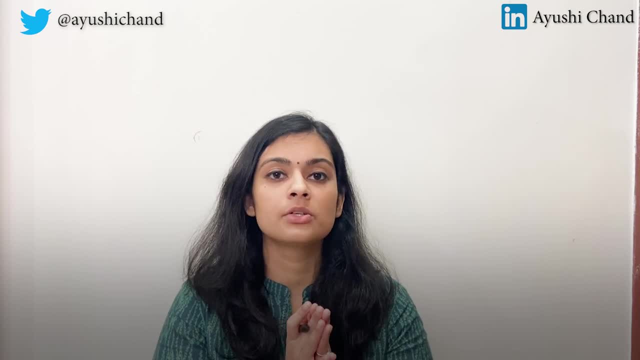 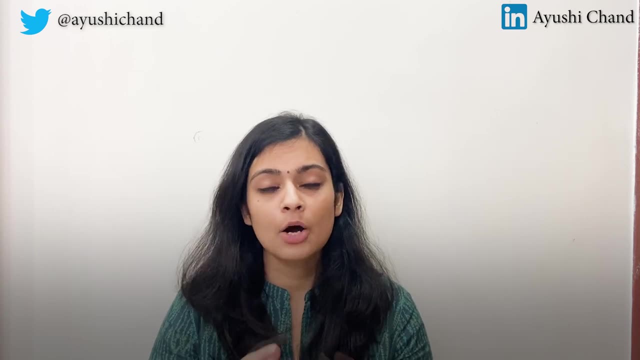 measured. So value chain is something which I discussed in part two of the series. So if you want to know more about value chain again, you can go to the link in the description box below. Basically, I discussed what causes prices to rise and how inflation affects our income. 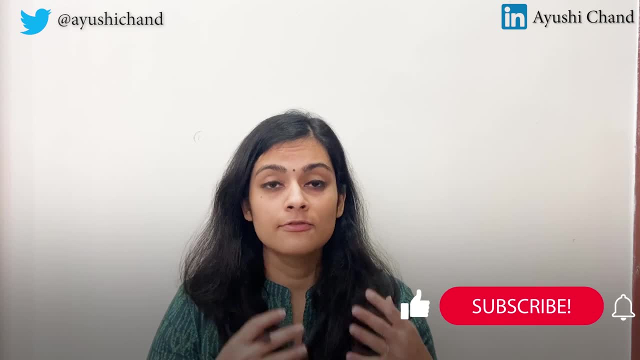 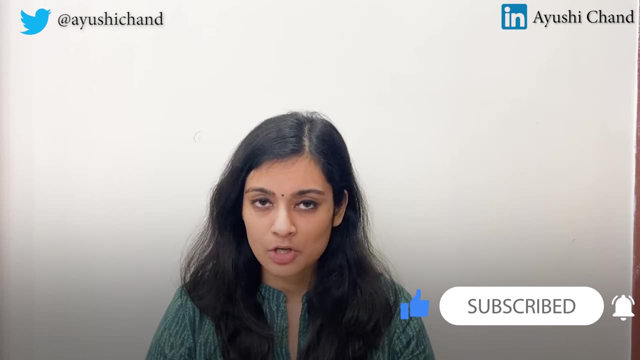 our savings, our long-term wealth creation and, in fact, inflation can be so dangerous that it can lead to the economic crumble of entire nations. So if you haven't watched that video already, do watch it right now, because it will give you an idea about how dangerous inflation can be. 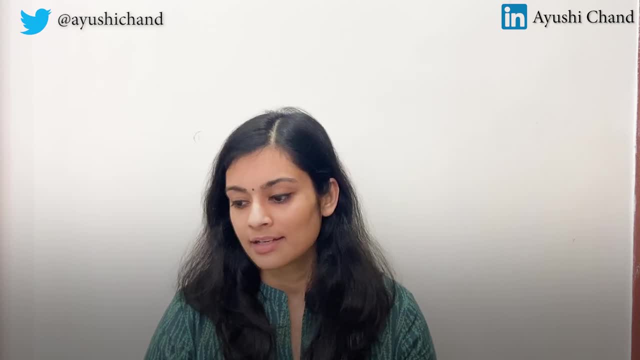 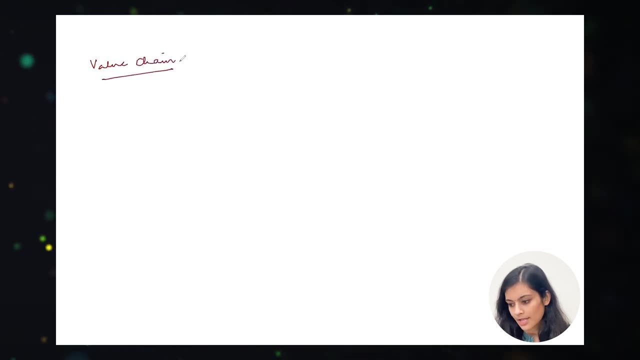 and what should we be doing to curb inflation? So let's talk about value chain again. Value chain is nothing but the production chain. It basically gives an indication of what all stages does a particular product go through in the production cycle. So let's consider the example of 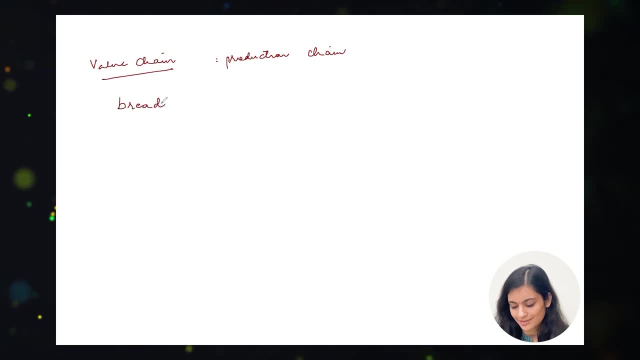 bread. Now a lot of people consume bread, So let's take this example now. Let's go back to the basics, where the producer is basically the farmer. So let's take this example now. So the producer is basically the farmer And then the farmer basically grows wheat. 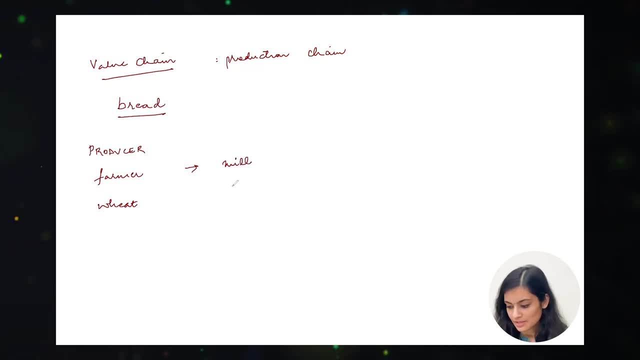 Farmer sells it to an atta, chukkiwala or the mill, wherein the mill converts the wheat into wheat flour. The mill owner then sells this product to a baker. The baker then converts the wheat flour into bread And finally, the baker sells it to the end consumer such as you and I. 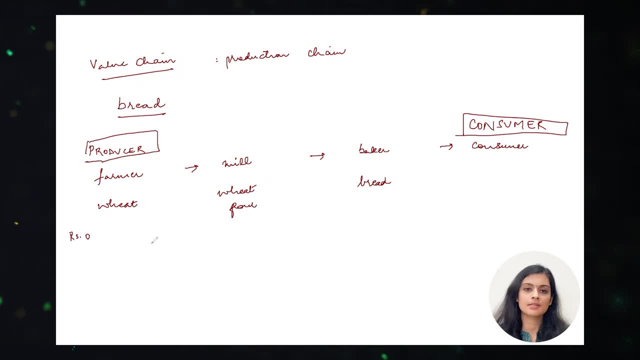 and we consume this bread. So when the farmer starts producing wheat, he's starting at zero. He takes some inputs, He'll take the seeds, He'll take fertilizers, pesticides, He'll grow the crop, He'll thrash, head, cut it and then finally add value worth rupees five and sell it to the mill. 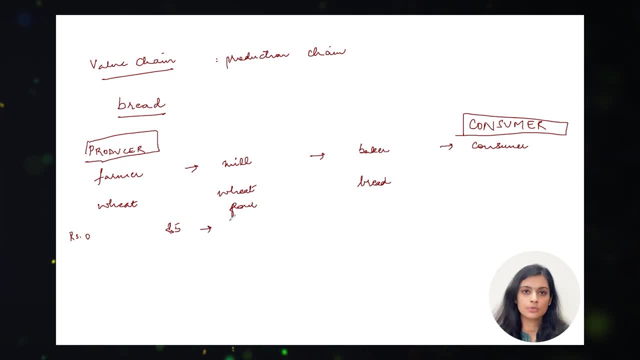 owner at rupees five. The mill owner is then going to take his equipments, which are the grinder, et cetera, and then he's going to grind the wheat into wheat flour and add worth to it and sell it, sell the wheat flour to the baker at rupees say, let's say 10.. The baker then adds value. 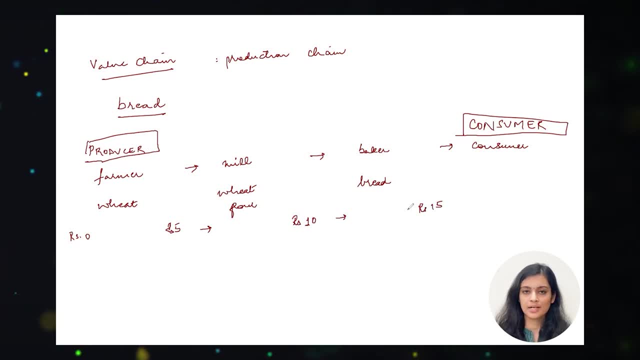 worth rupees 15.. He takes an oven, he bakes the bread and finally he sells it to the final consumer at rupees 15.. So we, as consumers, end up paying rupees 15 to the baker. Now there are three. 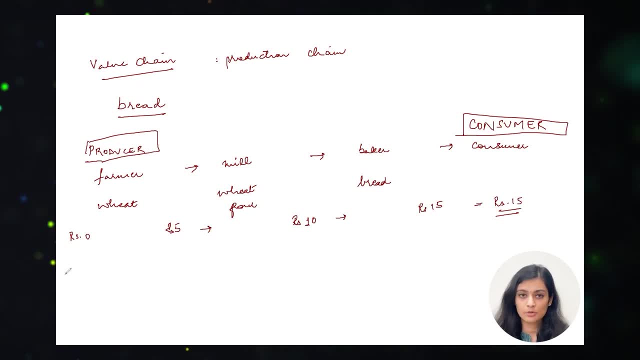 ways to determine GDP And with this simplified, oversimplified example, I'm going to cover all the three ways so that you have a broad understanding of how GDP is measured. The first way is called as value add approach. This basically sees what is the value being added at each stage of the 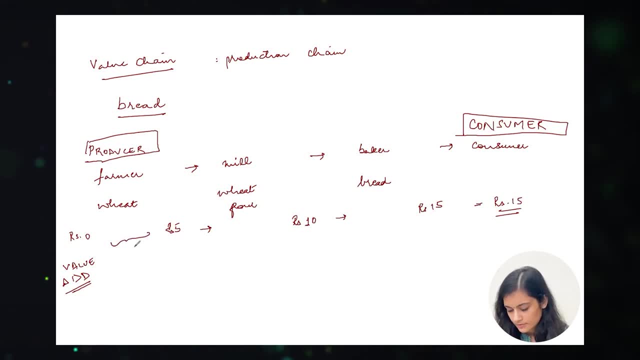 production cycle. So here let's see: the value add is rupees five, The value add at the mill owner stage is rupees five again. The value add at the baker stage is rupees five again, And finally we end up paying. 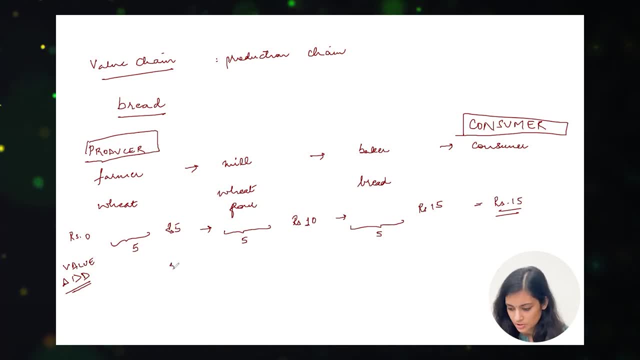 15 rupees. So if we look at the value add at each stage of the production cycle, here it is five plus five plus five rupees, And this means that the final value of the good is rupees 15.. This is the final value And hence, by the value add approach, the GDP of the country would. 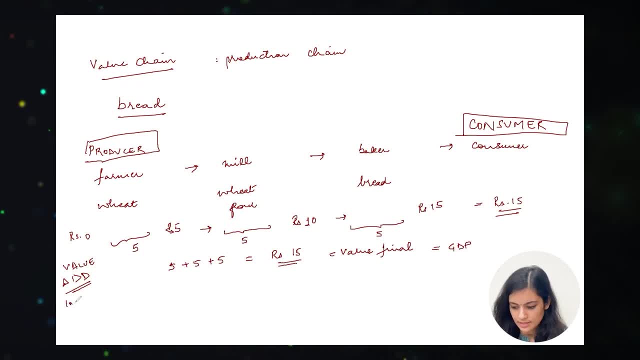 be equal to rupees 15.. The second method is called as income method. Now income method will see that what is the income that is being earned by each stakeholder in that production cycle. So let's say that the farmer has zero input costs and he earns rupees five out of it. 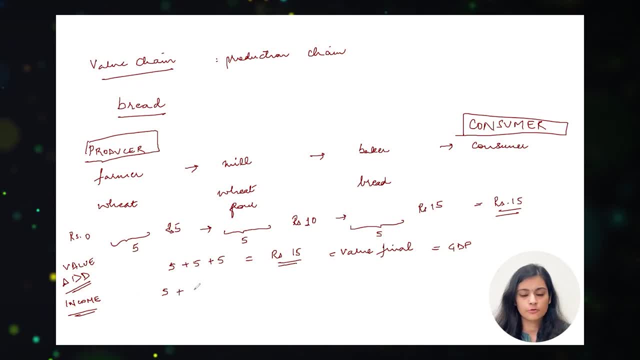 The mill owner purchases the wheat from the farmer at rupees five, So his input cost becomes five, and finally sells it at rupees 10.. So the income he's earned is rupees 10 minus five. Similarly, the baker is selling his produce or selling his product at: 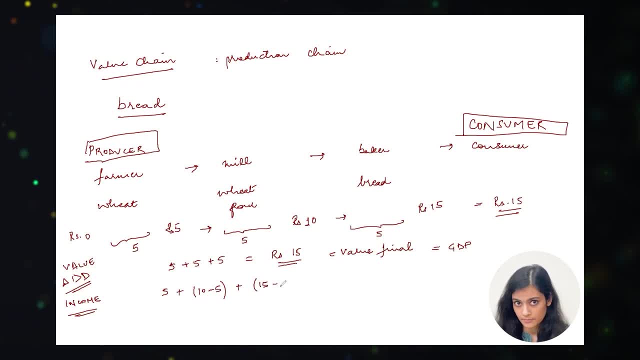 rupees 15, but purchasing the raw inputs at rupees 10.. So we'll subtract that from 15.. And this means five plus five plus five, again rupees 15.. This means again by income method, the GDP comes out to be rupees 15.. 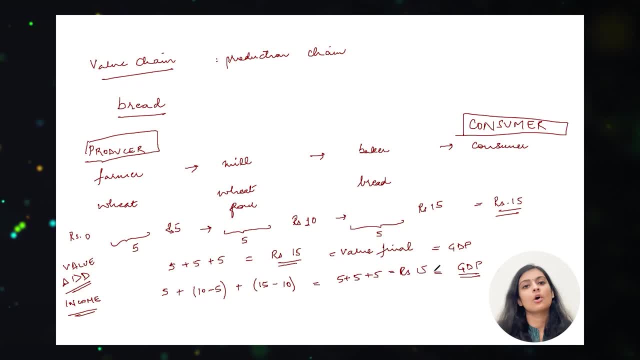 That means we are just taking the net income of all the stakeholders in the production. The third way and the most commonly used way is called as the expenditure method. This basically sees that what is the final expenditure being done by the consumer while purchasing that good? So it is a very, very simplistic measure in a way. So it says that 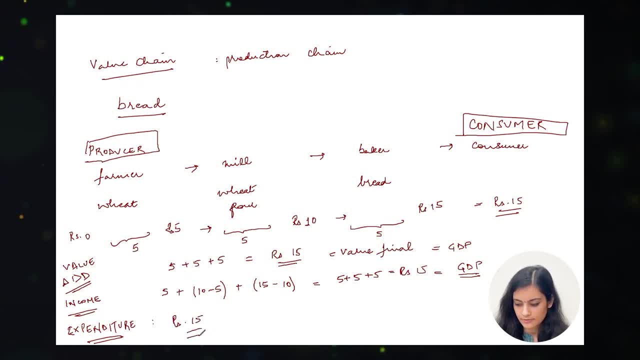 the final consumer is paying rupees 15 to purchase that final bread that we are consuming. So that's what it is. So, by the expenditure method, the GDP of the country would be rupees 15.. Very, very simple, right. So this expenditure method is the most commonly used method of GDP. 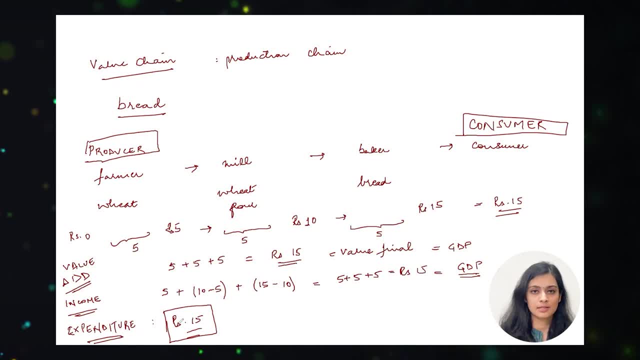 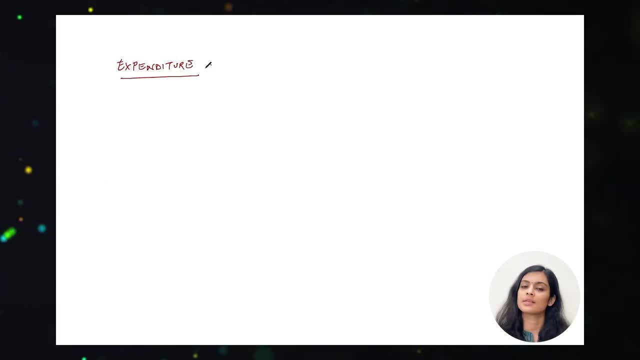 determination. So let's delve into the expenditure method in a little bit deeper fashion. So by the expenditure method we are going to make our example a bit more realistic. We are going to consider all the stakeholders that are involved in the economy So broadly. 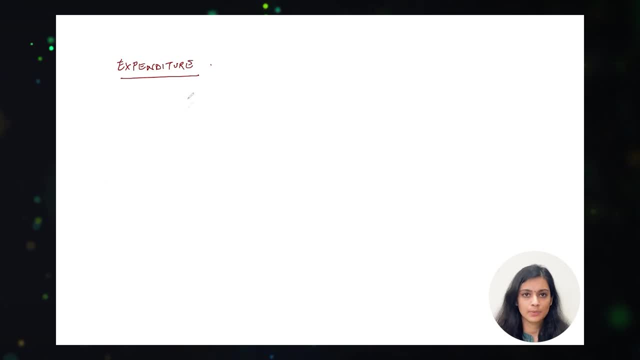 if you look at the stakeholders involved, it would be people like you and us, the final consumers, or let's call them the households, Because as households we tend to purchase a lot of goods and services. Then there are private firms, or the private industries, or the private companies. 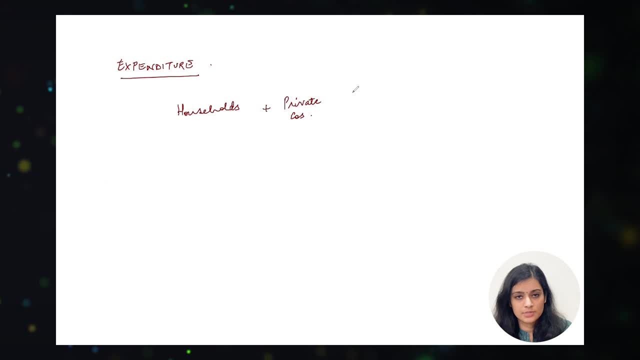 They purchase a lot of inputs for production of these goods and services. It could be heavy machinery, It could be capital equipment, It could be employing more labor, So all these would be counted as private expenditure. Then there is the government as another stakeholder. So government. 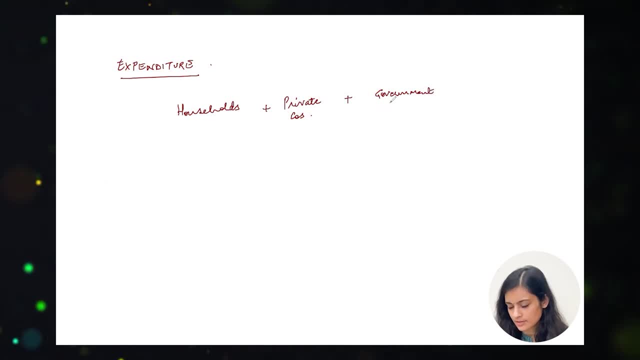 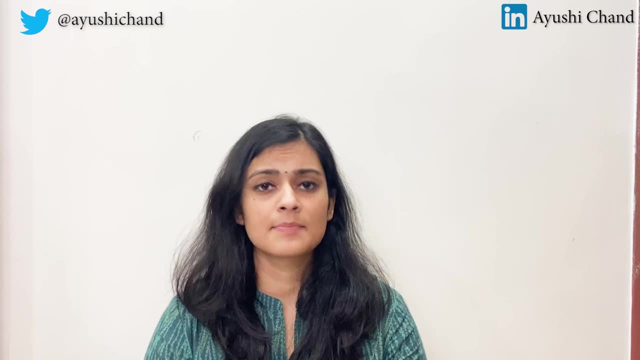 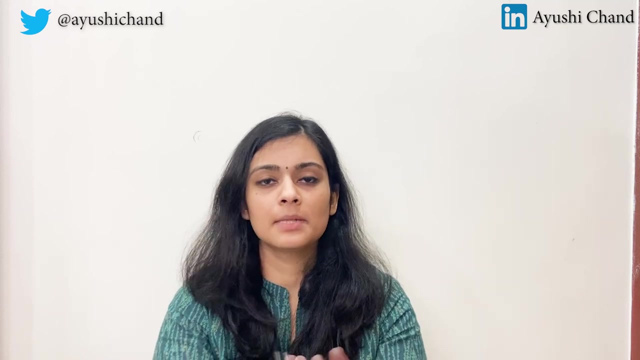 again purchases a lot of goods and services. So this could be giving the salaries to government employees. This could also be spending on defense, spending on infrastructure, creation of buildings for health, for education, and so on and so forth. So all these would be counted as government. 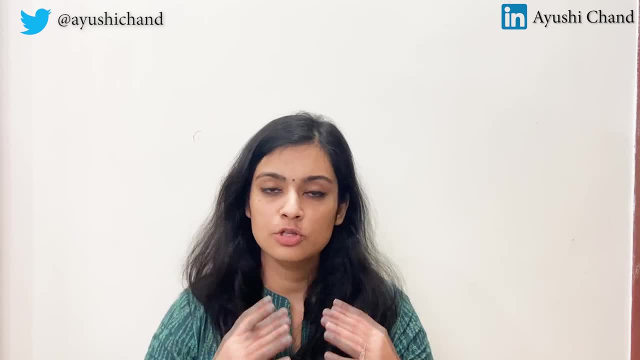 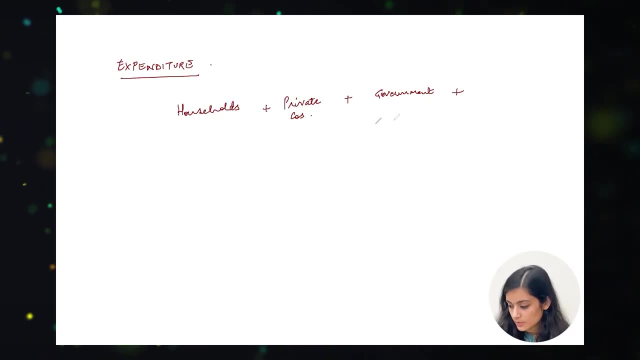 expenditure. And finally, a lot of goods and services are also exported out the country Because there is demand for these goods and services, which are produced in India, outside also. So we will also include the goods and services that are exported, but we will also 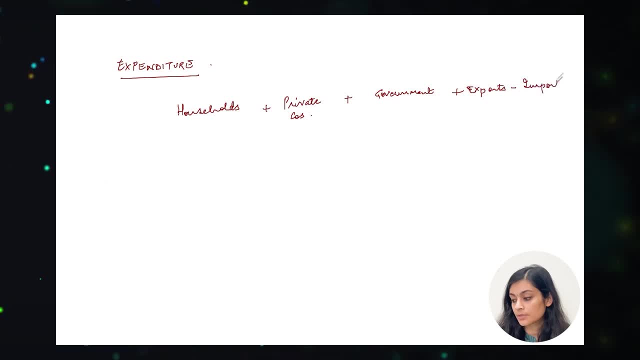 subtract the goods and services that are imported, that are produced outside but are imported in India. So exports minus imports would also be included here. So finally, GDP becomes a summation or sum of all these. Household expenditure would be called as C, Private expenditure is usually denoted as I, Government expenditure is denoted as G. 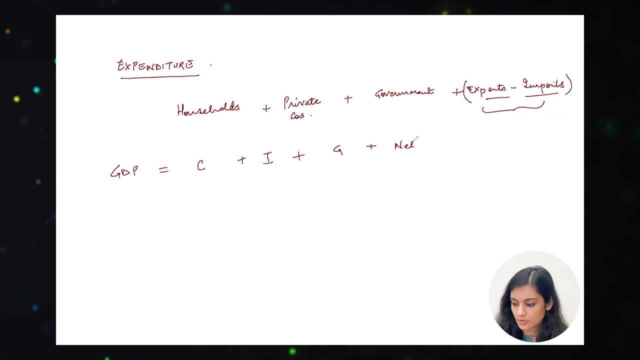 And export minus imports, also called as net exports, would be written as this netx. So this is one equation that you will see very commonly in textbooks across discussions which happen Even Raghuram Rajan. he gave an interview and he stated this particular definition there. 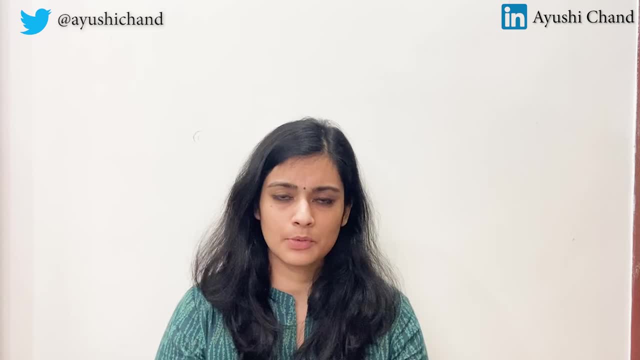 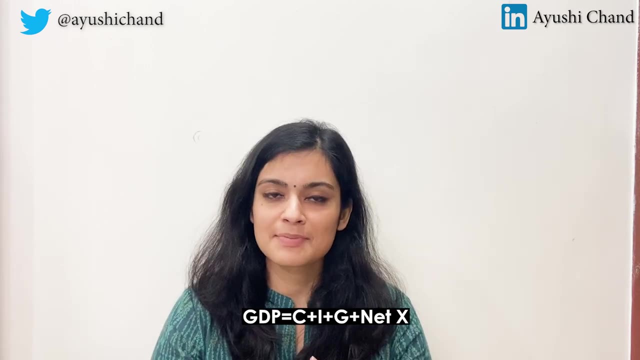 So this is something that you all might be familiar with. This is something that you all must know about because this is very, very frequently used. So GDP is a sum of household expenditure, of government expenditure, of private expenditure, as well as the net exports of the economy. With me so far, 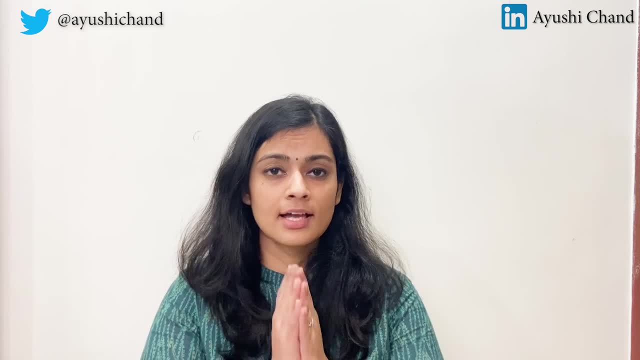 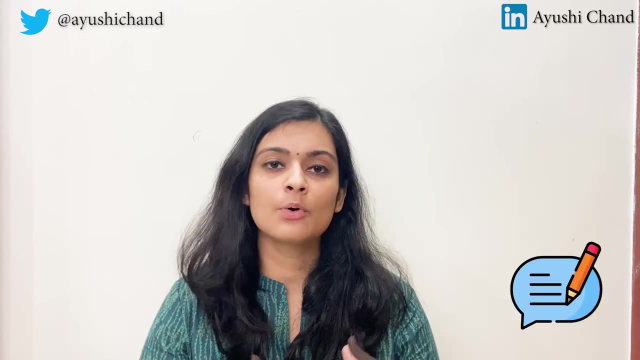 Now I have a question for you here. Do you think financial transactions, for example buying equities or buying bonds, is included in this calculation of GDP? Comment down with your answers in the comment box and I'll post my answer in the description box in a. 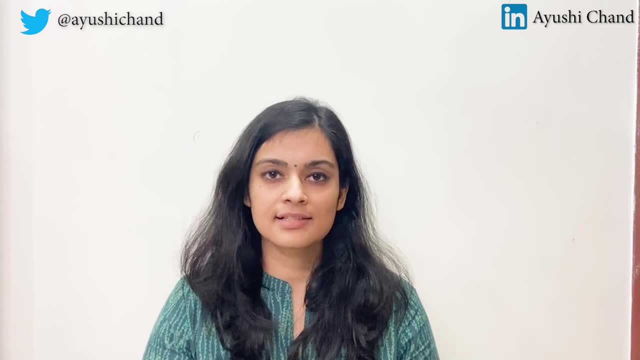 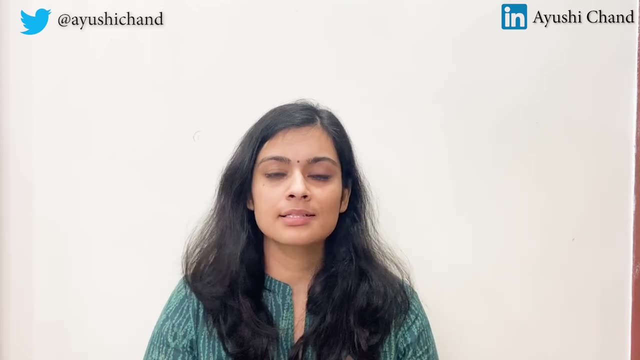 couple of hours Now. this was the theoretical or the more technical side of GDP. Let's come to the more practical aspects of GDP, wherein we discuss whether GDP is actually the right measure to understand the size or the health of the economy or not. Now let's take an example of country A and 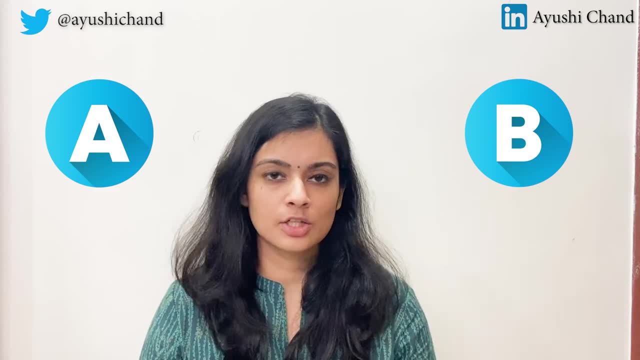 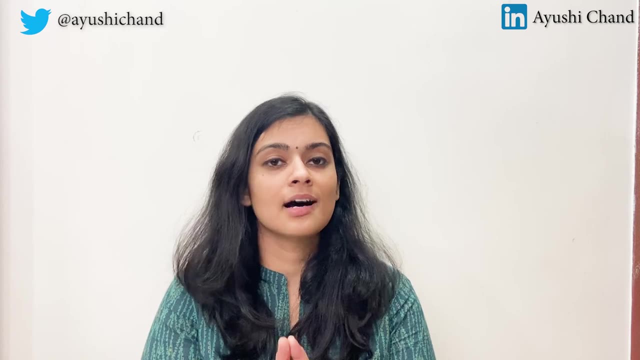 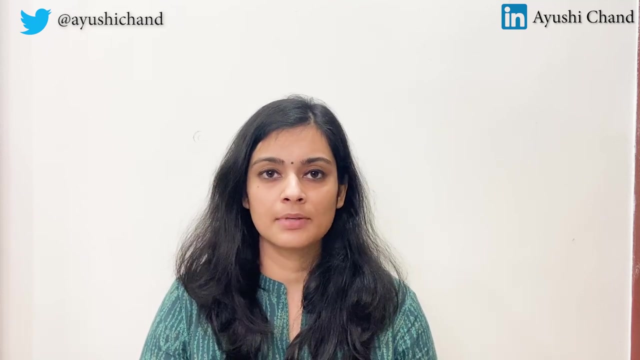 country B. Let's say country A has a GDP of $100 and country B also has a GDP of $100. Do you think they're at par with each other? Well, the answer is no. The first aspect that we have to consider is population size. Let's say US and China both have the same GDP, but do you think? 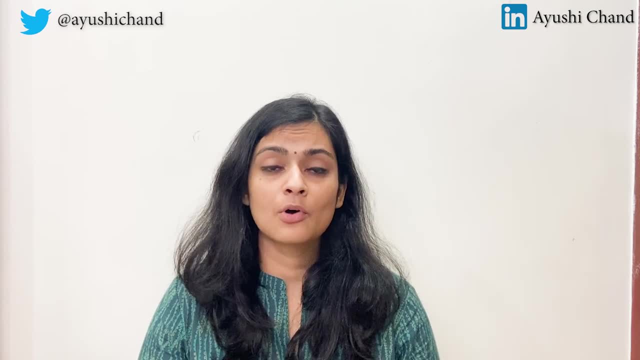 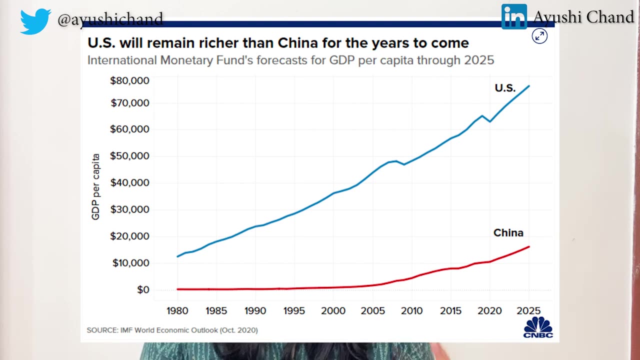 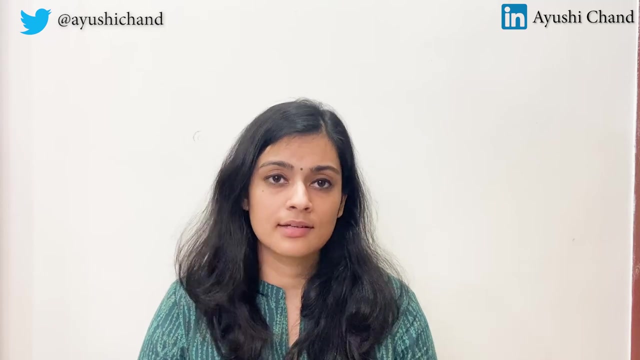 that they are at par with each other. No, because China has a population of 1.4 billion people. However, US has a population of only 300 million people, So that means that GDP per population or GDP per capita is not the same GDP per capita. 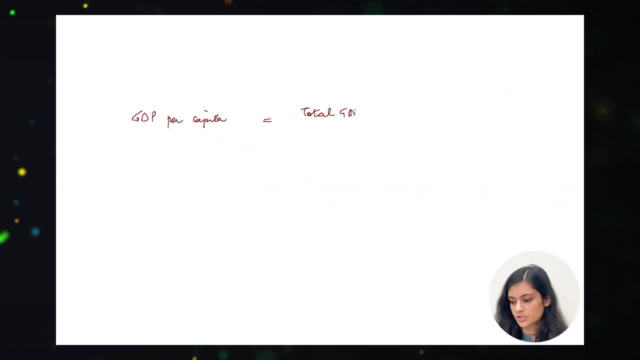 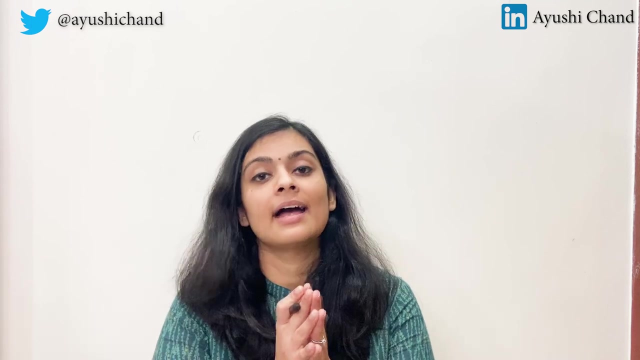 is basically total GDP of the country divided by total population of the country. So, while the GDP of two countries may be the same, but if the total population varies, then the GDP per capita or GDP per population will vary, and hence it will give a very, very 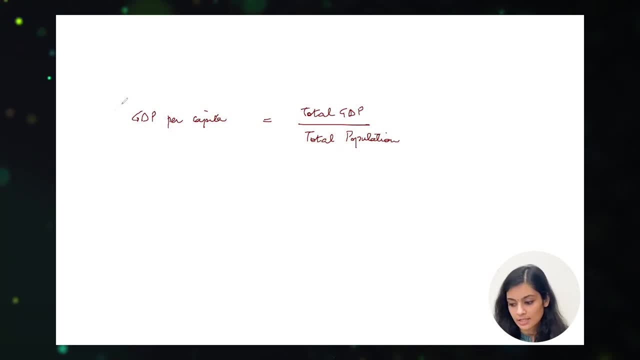 different picture about the two economies. This is one thing that we must always keep in mind, So comparing just the GDP of two countries is not the right way to go about it. The second aspect that we have to look at is GDP growth rate. 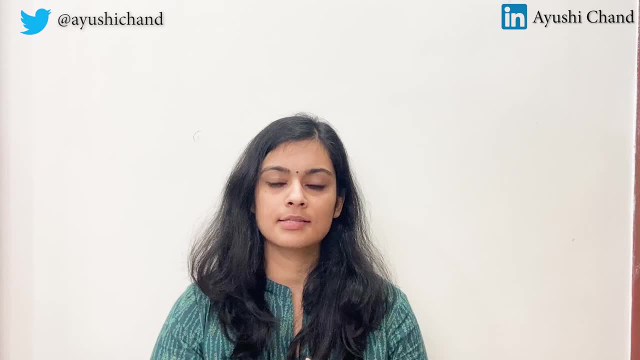 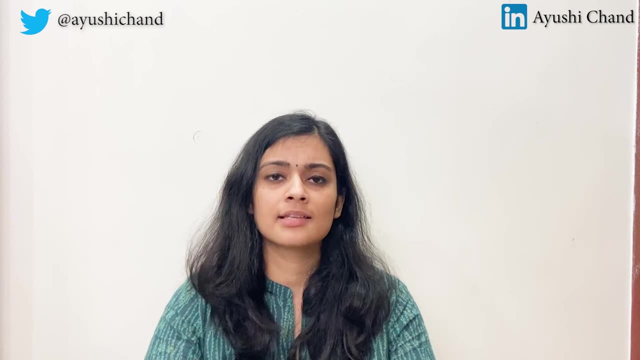 Now, because the state of any economy is very, very different from other economies. so no two economies would be the same. They might be similar, but the nature of the politics there, the nature of the goods and services that are produced there, the kind of production that. 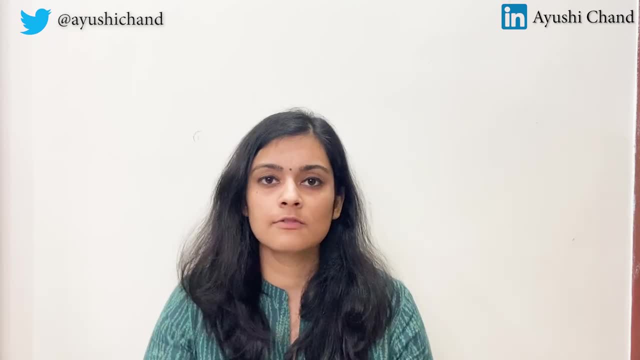 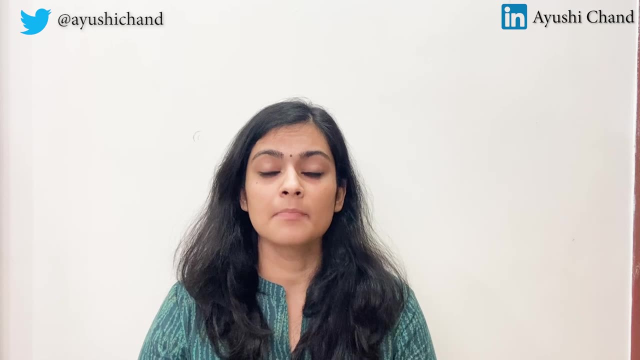 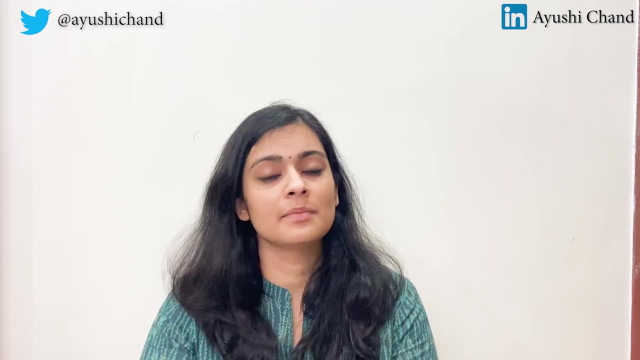 happens. the dependence of that economy on external factors might be very, very different and hence the GDP of two countries may not be comparable. So we must look at the growth rate of the GDP. Growth rate measures the change in GDP which happens in that particular economy itself. So, for example, if we say that India is growing at 7%, 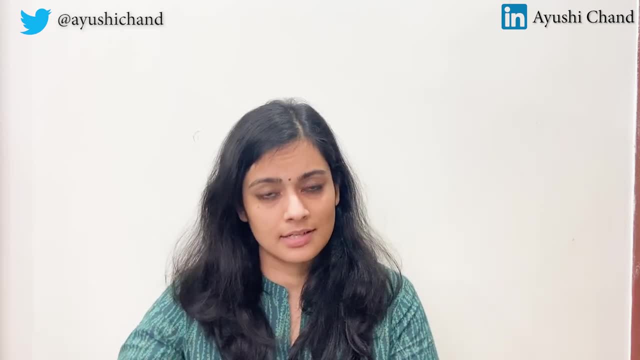 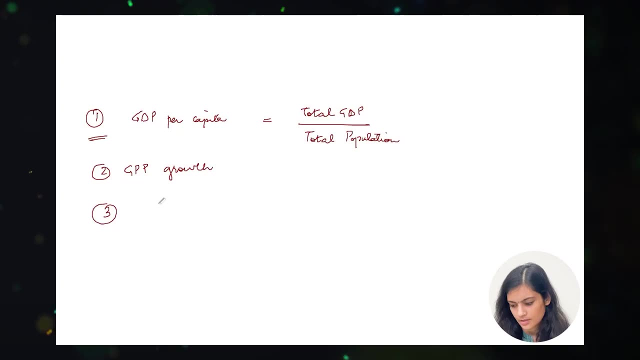 it means that the GDP of the country is increasing at 7%. So therefore, GDP growth rate becomes a better measure to calculate the actual progress that is happening in the economy. The third aspect is something called as purchasing power parity, A very, very current concept. to understand, the concept of purchasing power parity basically states that 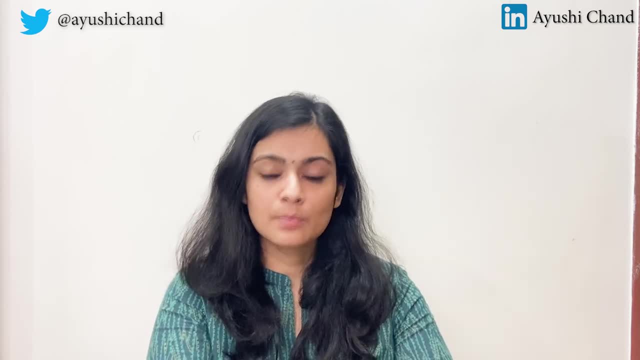 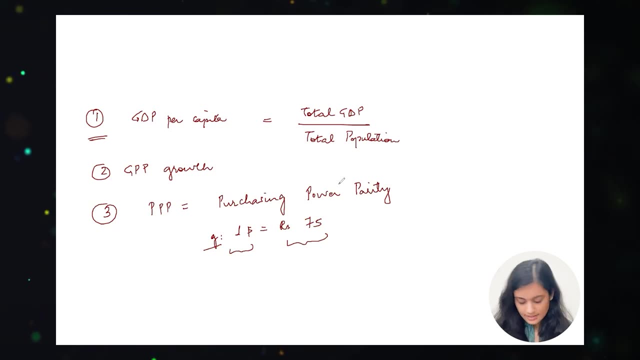 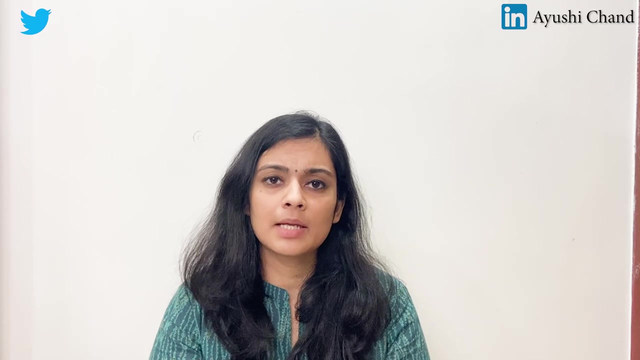 the value of the goods and services that we can consume in one country may not be the same in another country. if we look only at the exchange rate. For example, let's say that the exchange rate of US Dollar to INR is: one dollar is equal to Rupees 75. But do you think we'll be able to consume the same? of goods in one dollar in USA as in rupees 75 in India? Definitely not, because the cost of living in India is much less than that in USA. For example, there is something called as Big Mac Index which is used to compare the cost of living in different economies. The idea is simple. What? 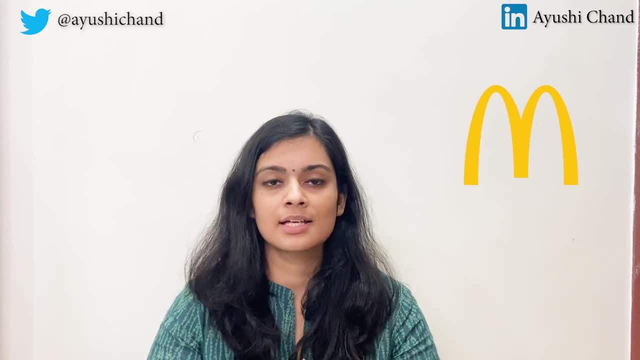 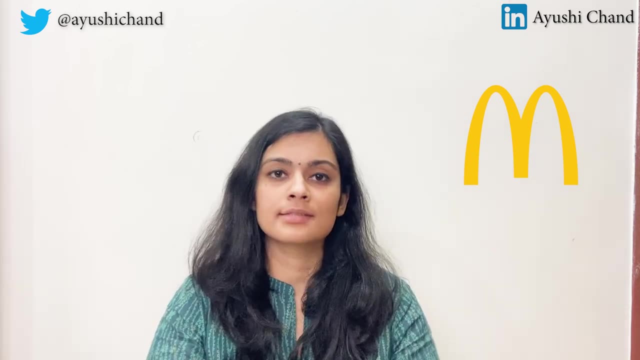 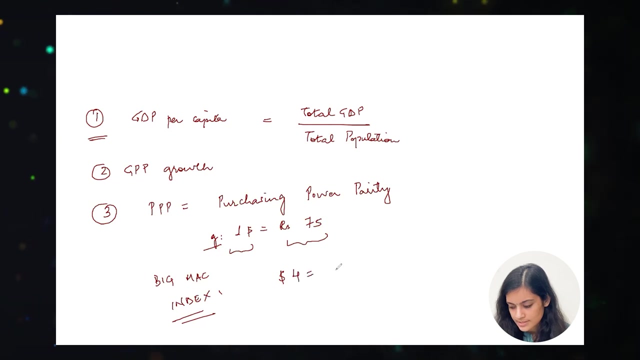 it says is that McDonald's is a chain which is committed to consistency. It uses the same raw materials, It uses the same technique to make burgers across the 120 countries it is present in. So a burger which costs dollar 4 in USA, which, if converted into rupees, would be approximately. 300 rupees. Do you think that we will get same burger, same one burger, in India at rupees 300?? No, we can in fact get 6 burgers here. So while in USA, let's say, we were able to purchase only one burger, here we are able to purchase 6 burgers. 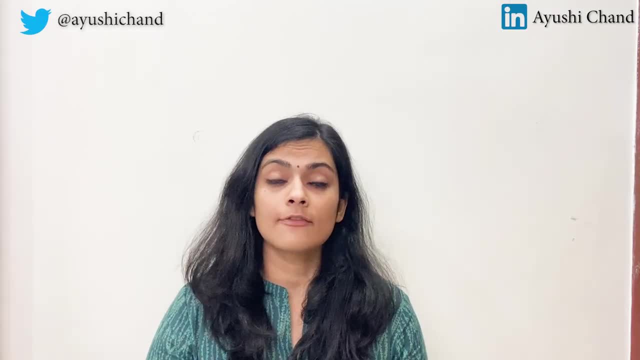 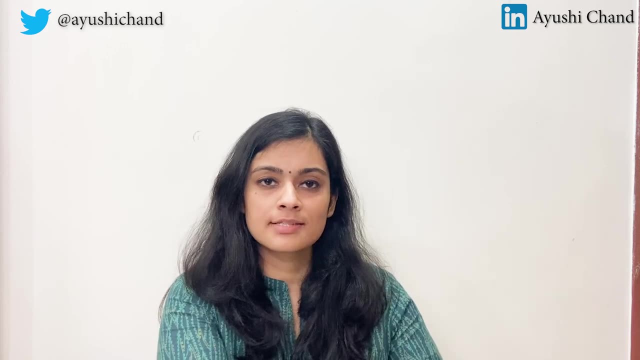 So this is basically PPP. So we have to do an apple to apple comparison. We have to see what is the real exchange rate at which we can actually purchase the same amount of goods and services in country A vis-a-vis in country B. So, while the exchange rate may be one dollar is equal to rupees 75, but in purchasing power parity terms it may not actually be true. It may actually be extreme. So what we are able to purchase in one dollar in USA, we may be able to purchase the same. 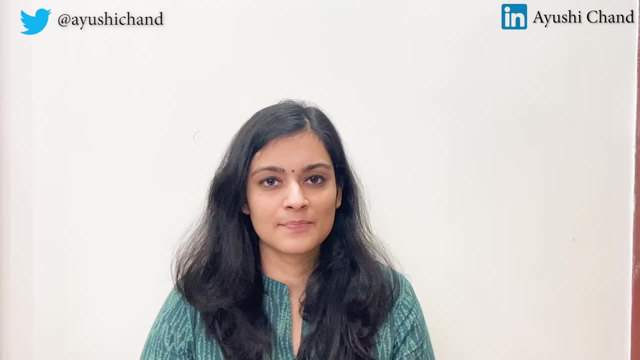 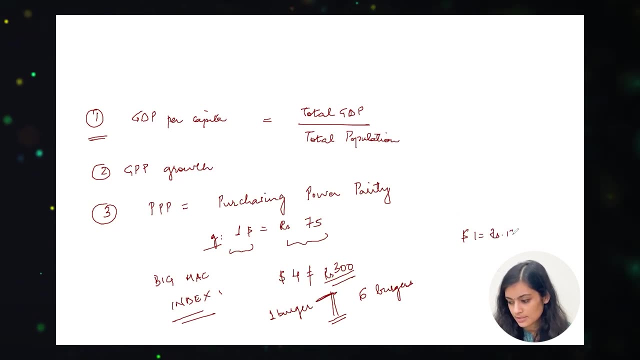 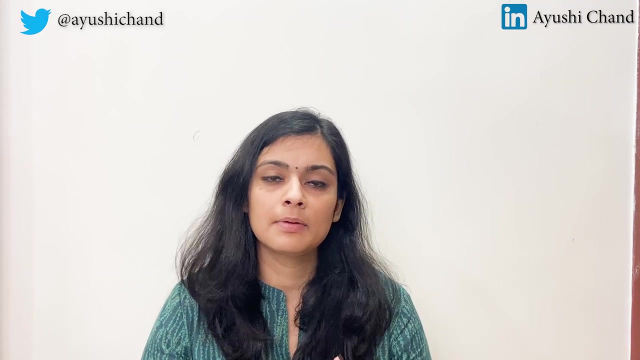 amount of goods and services in 12 rupees in India. So the actual exchange rate in PPP terms may actually be: one dollar is equal to rupees 12, and this is what the concept of PPP is all about. The problem here is that PPP is very difficult to measure. First, it is not that the same. 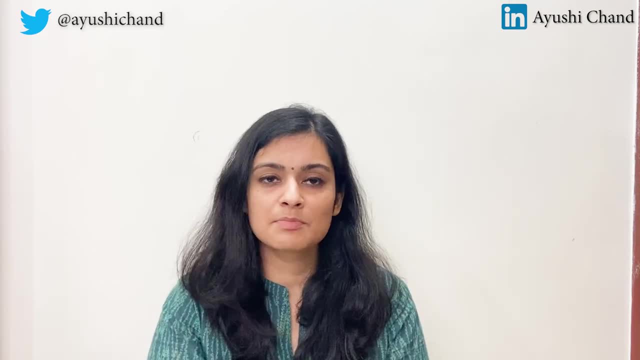 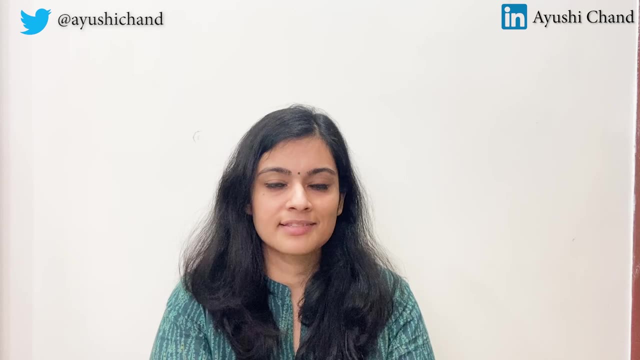 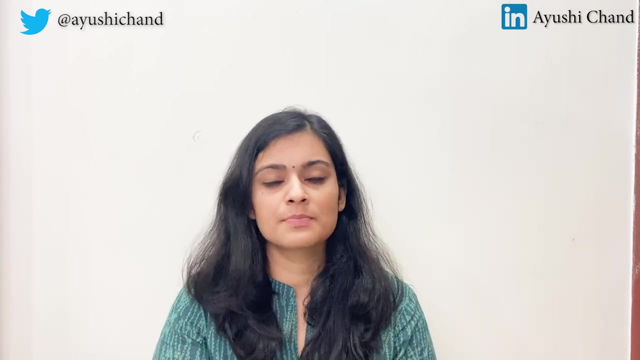 basket of goods would be consumed. The preferences may vary, The kind of product that are consumed may vary, So it becomes difficult to actually see what is the basket of goods that should be compared across different economies. So Big Mac Index was one estimate that was introduced by University of Pennsylvania. 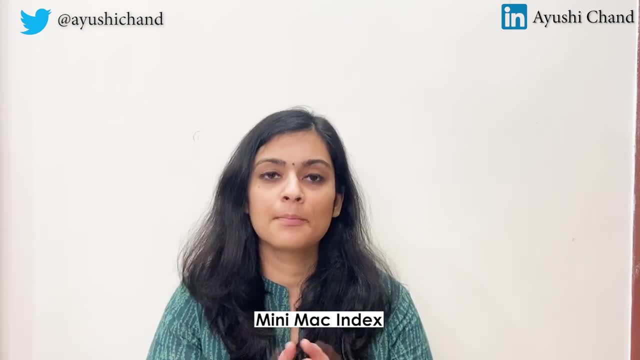 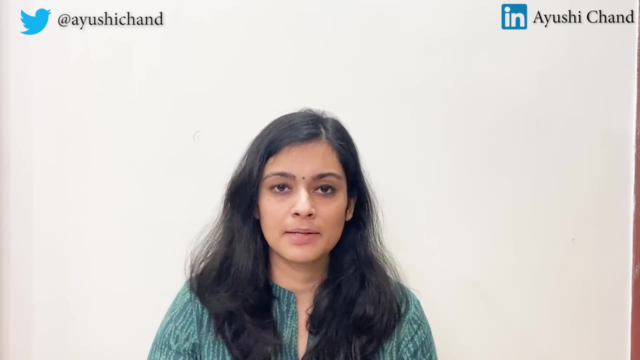 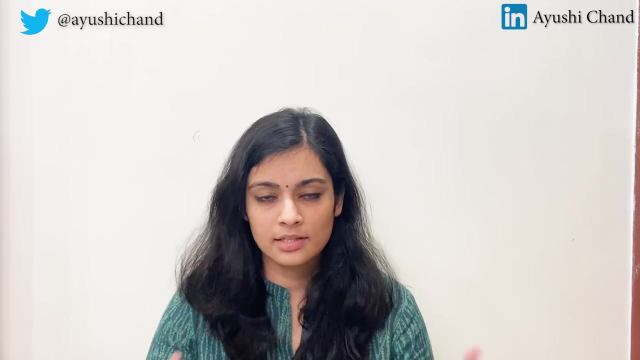 There was also a Mini Mac Index which was introduced, which basically compared the prices of a mini iPad across different economies and then estimated the exchange rate in PPP terms. There is a large faction of economists which says that GDP comparison across economies is not the right measure. GDP should actually be measured in PPP terms. So this is one. 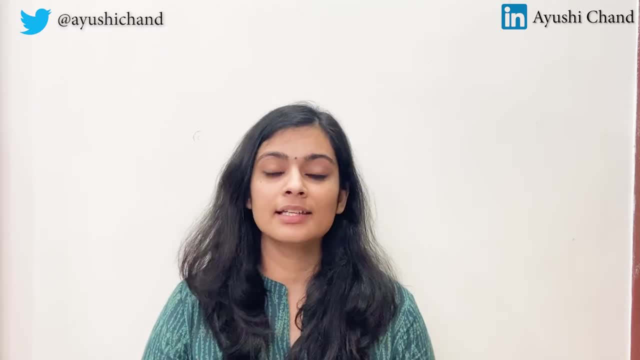 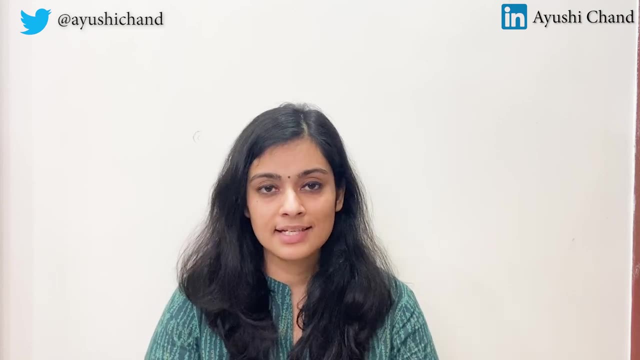 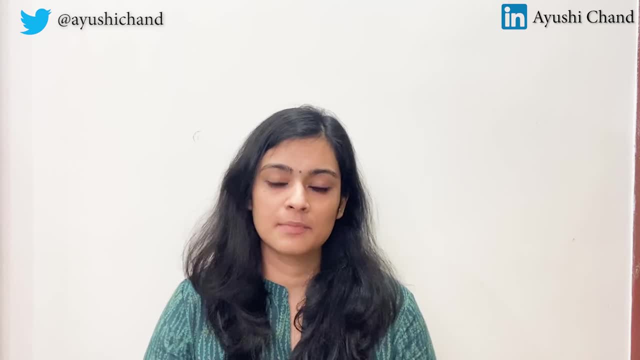 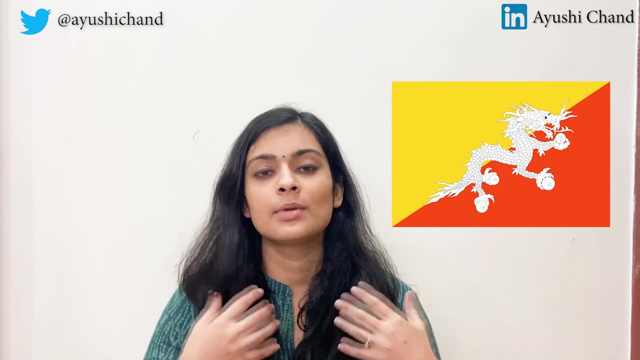 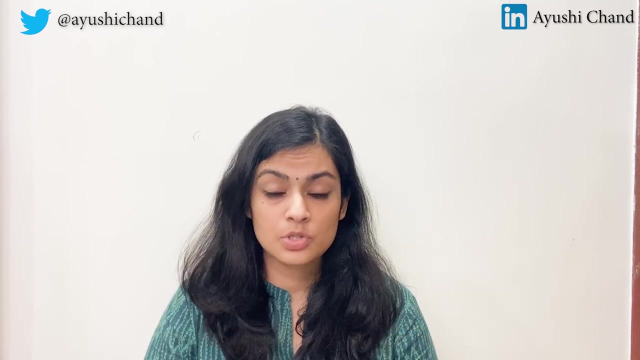 to be not an ideal solution to measuring how the economy is performing. let me give you a very interesting example here. Bhutan is one country which has come up with an index of its own. it is called as gross national happiness. now, gross national happiness is a multi-dimensional approach. 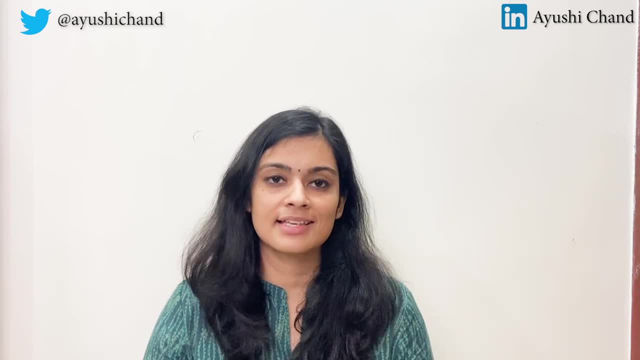 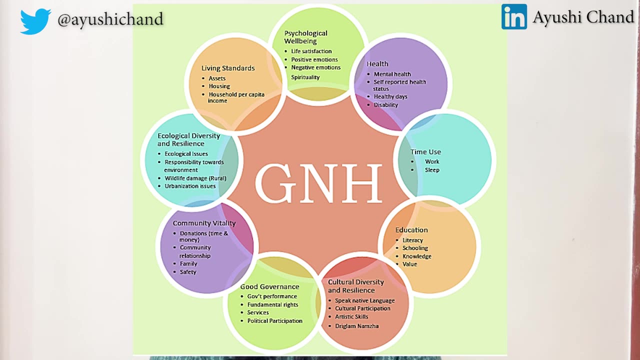 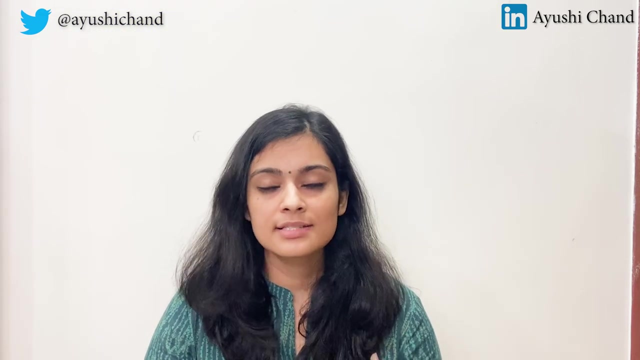 which looks at different indicators to actually assess the well-being of its population. for example, it looks at the psychological well-being, it will look at environmental factors, it will look at the education level, the health level of its citizen. it will also look at the sleep level, the community values and the governance of the entire economy and hence gross national. 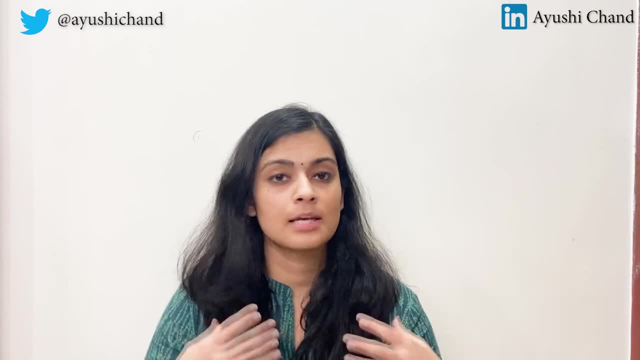 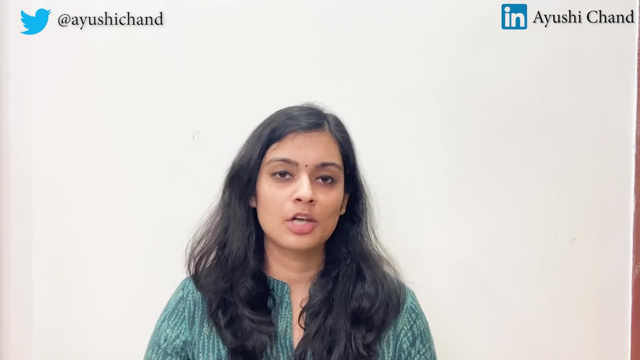 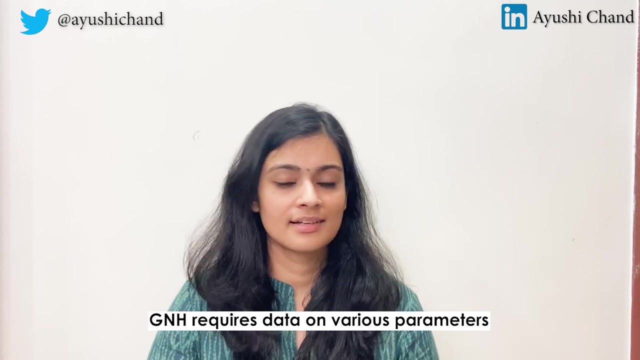 happiness is a very, very comprehensive index that Bhutan has come up for its own economy. now, whether such an index can be adopted across different economies is a very, very important, is a debatable question, because this kind of an index requires data on various parameters. various parameters such as health, education, such as good governance, ecological factors, sleep. 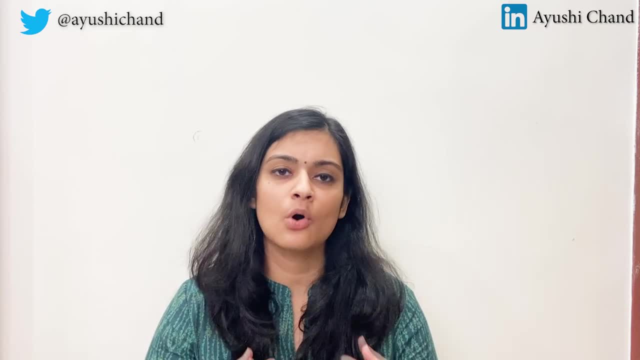 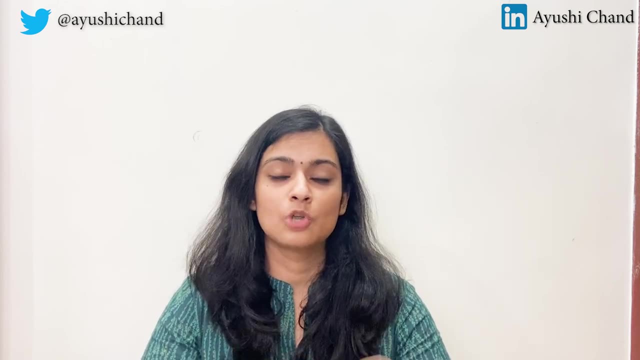 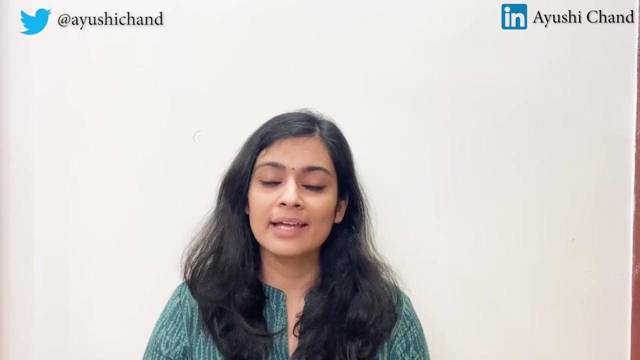 family values. now, these are something which are not always quantifiable, and hence it becomes difficult to come up with such an index and be adopted across different economies. I hope, with this video, you could understand what is GDP, how it is calculated, why it acts as an economic barometer to understand the size of any economy. I also discussed the 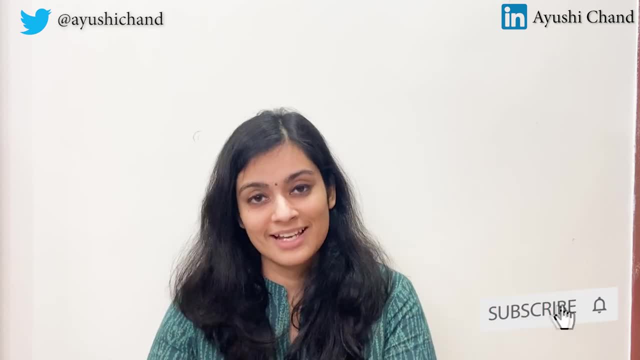 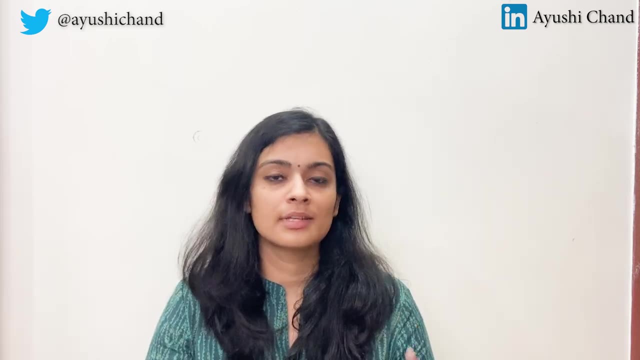 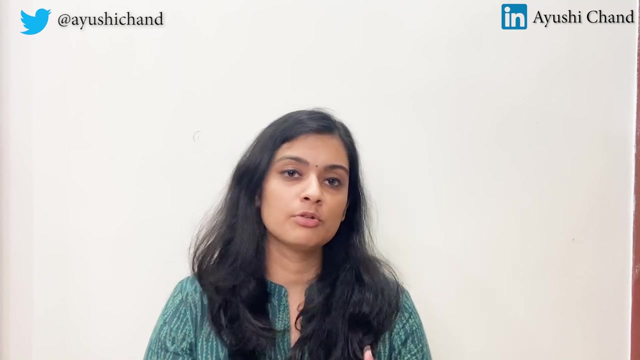 shortcomings of GDP and what could be an alternative index to actually assess the well-being of any nation. it is difficult, but that should be the road that all the economies should be taking now. I wanted to dedicate an entire video to GDP, because GDP is something that I'm going to discuss in my subsequent videos as well. GDP forms the basis of different 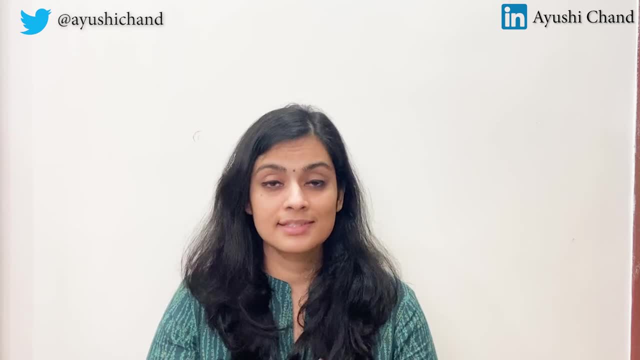 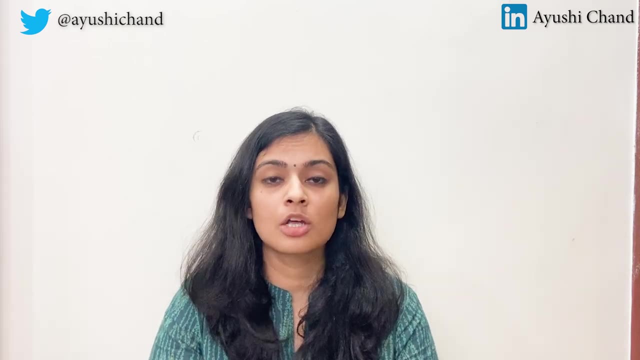 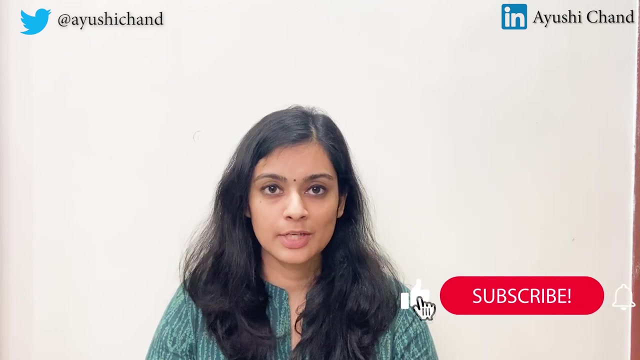 financial factors, different economic indicators, such as debt to GDP ratio, how it can actually prove as an indicator towards assessing whether an economy is going to perform well or whether it is going to default, and this is what I'm going to discuss in my next video. so please stay tuned. 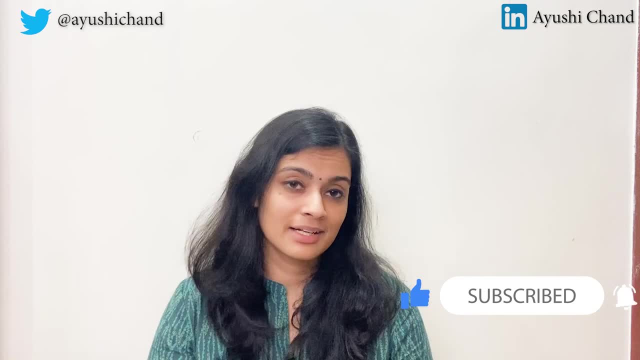 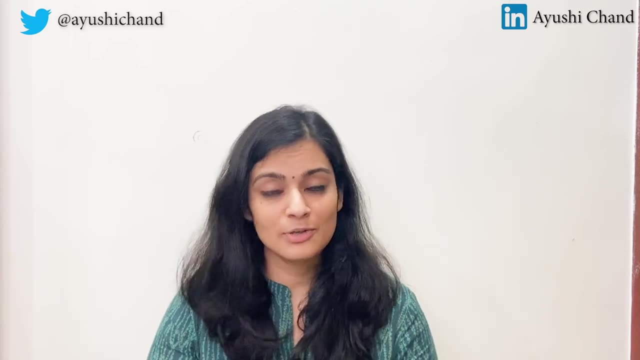 if you like the video, do press the like button. if you like my content, then please do subscribe to the channel. I'll be posting more content around economics and finance and all the other things, and also public policy. see you the next time. till then, stay safe, take care. bye.